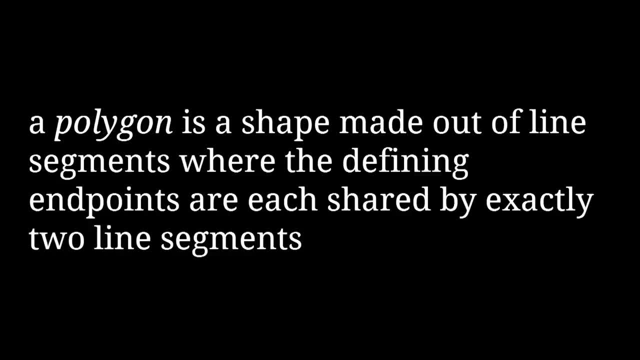 an example of a polygon. it's a polygon because it's made out of line segments, and all of the points that define the component line segments are shared by exactly two line segments. the points in a polygon are called its vertices and the line segments are called its edges. polygons can have 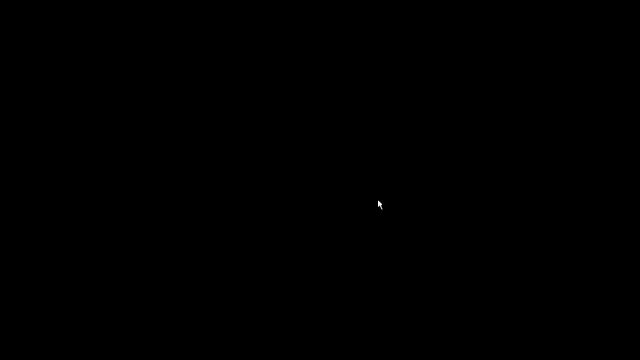 however many edges you want, as long as there's at least three. I mean you could have two of them, but they'd end up just being in the same place and the shape you end up with is indistinguishable from if you just had one line segment on its own. so that's usually not allowed. polygons can pretty. 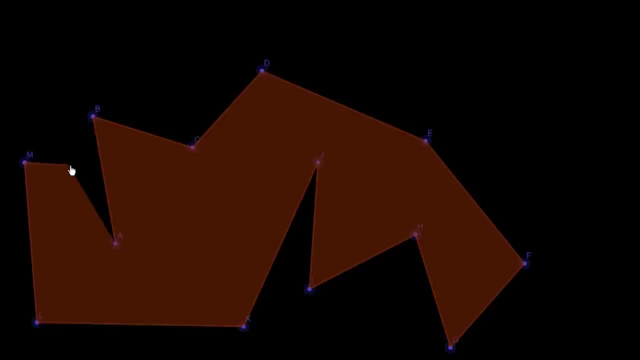 much be shaped however you want, as long as they fit the definition of being made out of line segments and every vertex being connected to exactly two edges. there's a special category of polygons, called regular polygons, which have a couple of specific properties that other polygons. 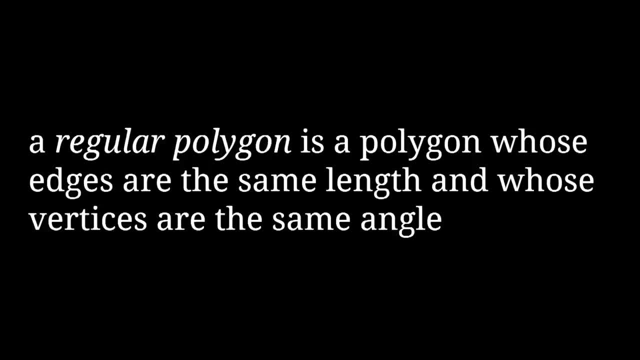 don't all of their edges are the same length and the vertices that they meet at all have the same angle. this is an okay enough way to describe what it means for a polygon to be regular, but for my purposes it'll be useful to define these qualities a bit more precisely. for a 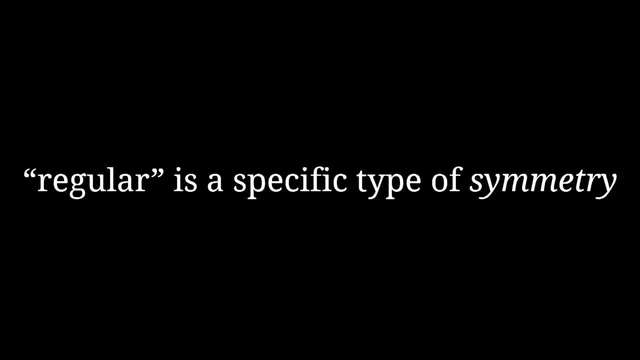 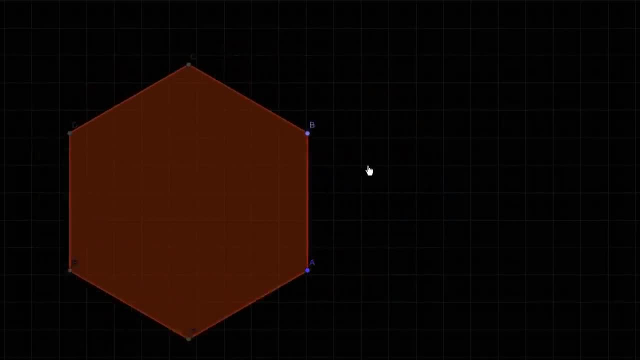 polygon to be regular, it must have symmetry, meaning that it looks the same in multiple different orientations. specifically, you have to be able to move any edge to any other edge or any vertex to any other vertex. these qualities are called edge transitivity and vertex. 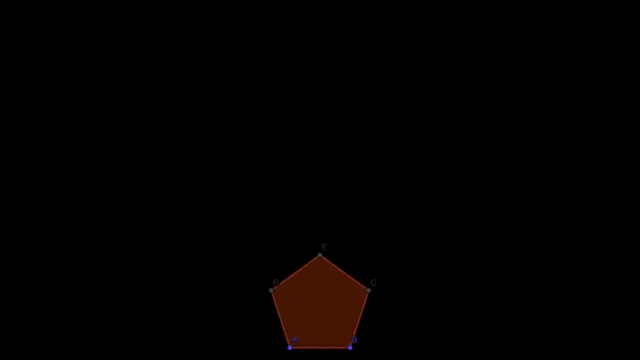 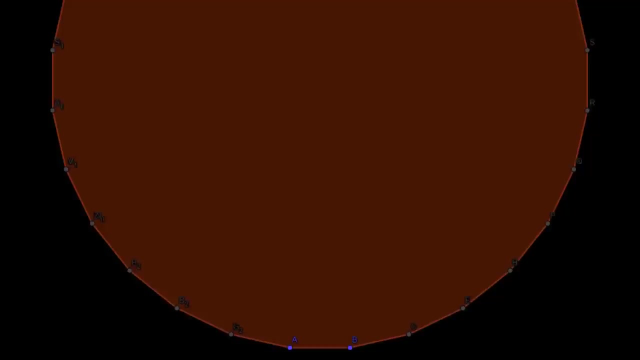 transitivity. there are infinitely many polygons that satisfy both of these properties and, in fact, you can construct a regular polygon with an arbitrarily large number of sides- triangles, squares, pentagons, hexagons, heptagons, octagons and so on- with no upper bound. on how many sides? 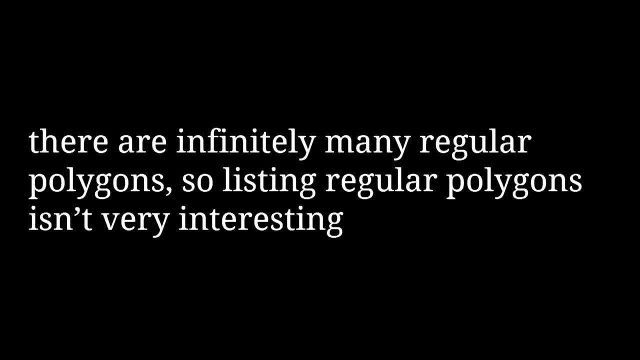 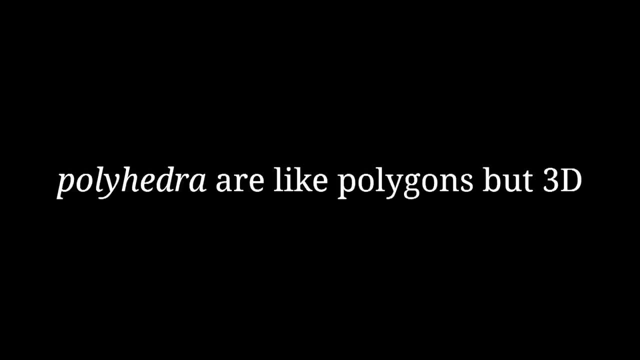 it can have. the fact that there are infinitely many regular polygons means that regular polygons are boring, so let's move on. the three-dimensional equivalent to polygons are the polyhedra. just like how polygons are made out of line segments, polyhedra are made out of polygons. 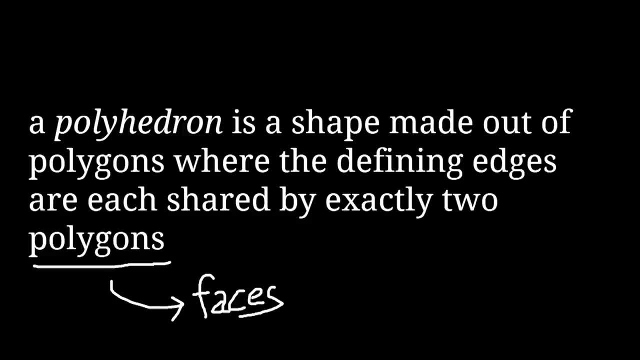 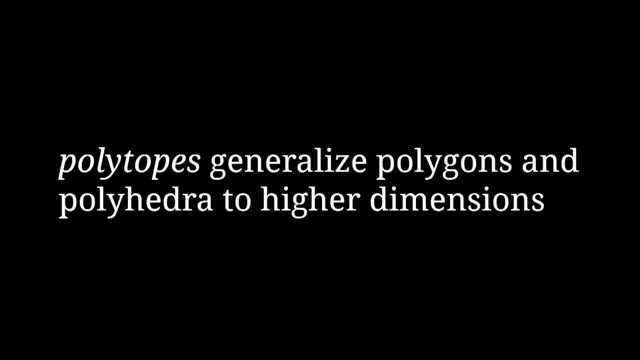 with each edge shared between exactly two of them. the polygons that make up a polyhedron are called its faces. polyhedra and polygons both belong to a larger class of shapes called polytopes, which generalize the concept to higher dimensions. higher dimensional polytopes are great. 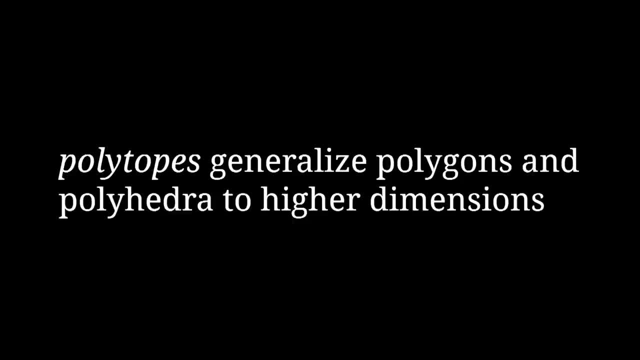 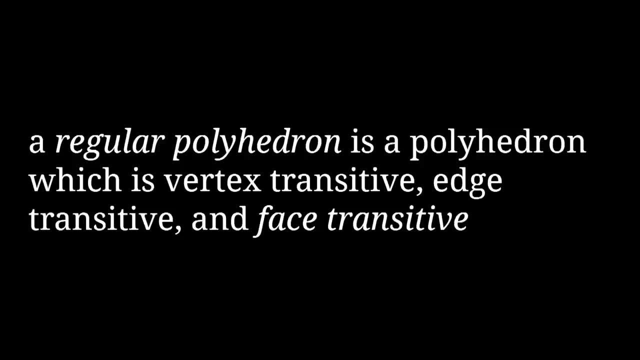 but this video will be entirely focused on shapes that work in 3D space, and the definition of regular polygons can be extended into a definition of regular polyhedra. once again, it's defined according to symmetry. in addition to vertex and edge transitive, a regular polyhedron must also be face transitive, so you can move. 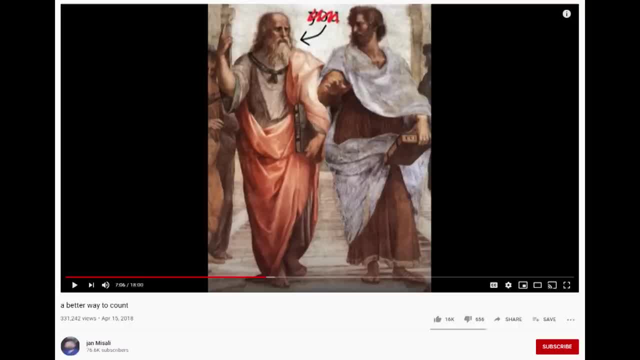 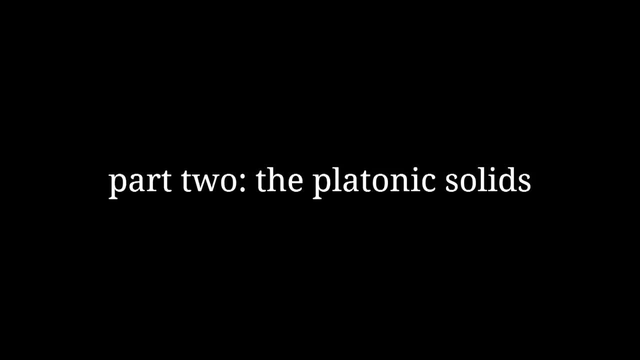 any face to any other face. the philosopher Plato showed that there are five 3D shapes that fit this definition, which are known as the platonic solids. okay, got all that great. part two: the platonic solids. the definition of regular polyhedron is pretty strict. 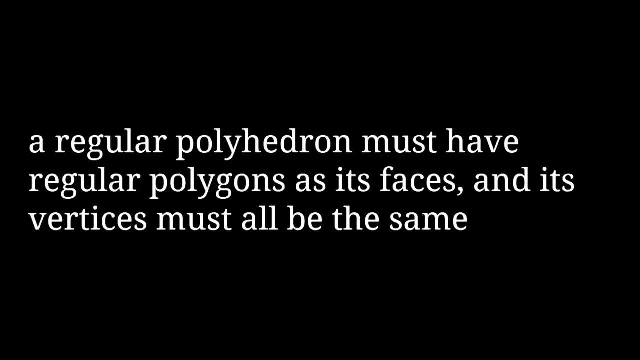 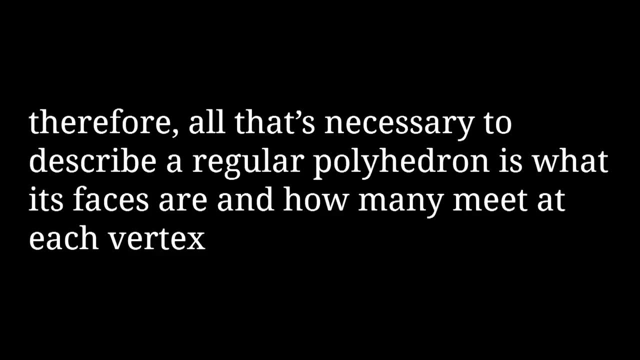 so it makes sense that there would only be five of them. I think it's pretty trivial to see that for a polyhedron to be regular, its faces must all be regular polygons, and for it to be vertex transitive, all of its vertices must be the same. so all you need to describe a specific regular 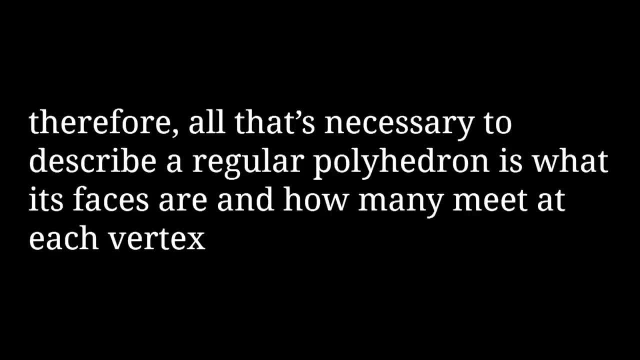 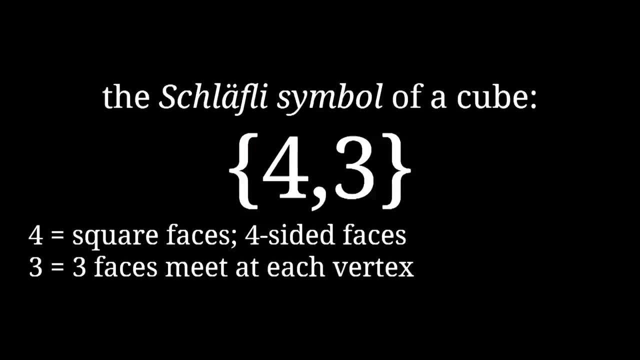 polyhedron is what shape its faces are and how many meet at each vertex. you can represent this information using a Schlafly symbol, named after Ludwig Schlafly, with the number of edges of each face, then the number of faces that meet at each vertex, all within curly brackets. okay. 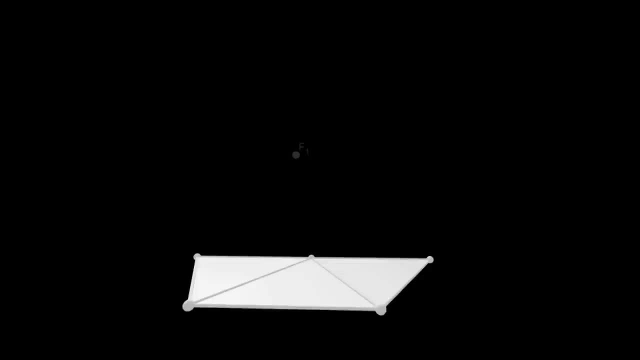 let's look at some regular polygons and see what regular polyhedra you can make out of them. if you start with three triangles and fold them up into 3D space so that they all meet around a vertex, the space remaining is perfect for one other triangle and you get a tetrahedron, also known. 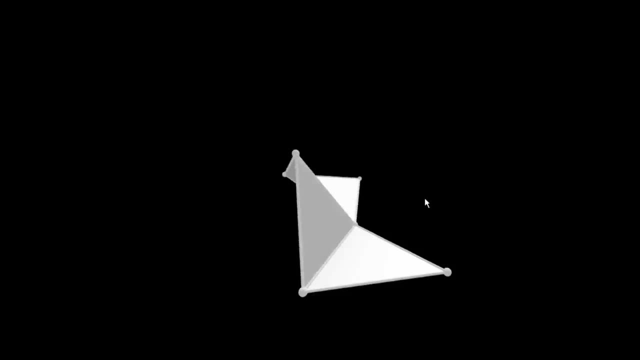 as a triangular pyramid. next, start with four triangles around a vertex, since you know each going to have to be the same. constructing any given platonic solid means looking for openings and putting in more faces, copying whatever vertex you started with with four triangles around a. 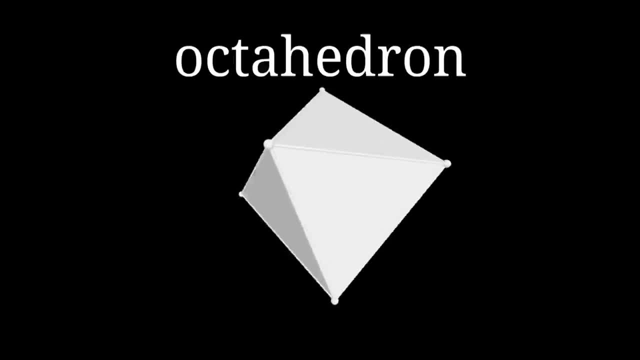 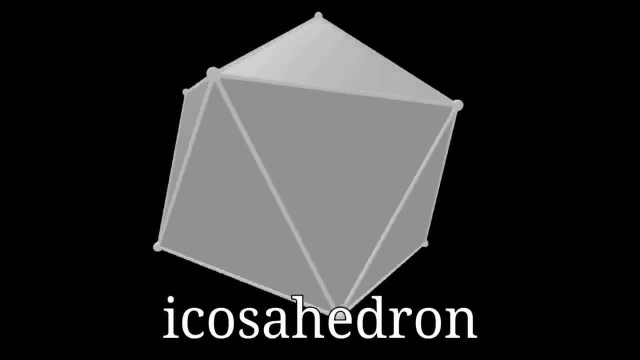 vertex, you eventually form a shape made out of eight triangles, an octahedron. doing the same thing with five triangles, you eventually get the lovely 20-sided icosahedron which you might recognize as a d20.. if you start with six triangles, you run into a problem: they can't. 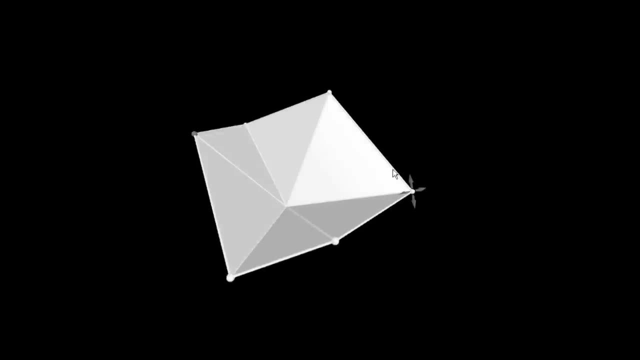 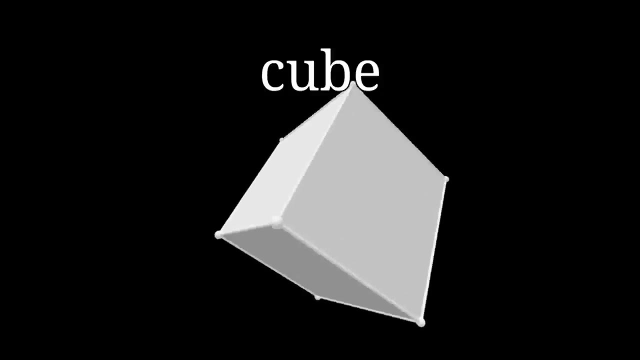 actually fold into 3D space because they lie flat. so you've now reached the point where you have too many triangles to make a platonic solid, so let's move on to squares. three squares around a vertex gets you a cube, and four squares around a vertex is too many because they lie flat again. last one: 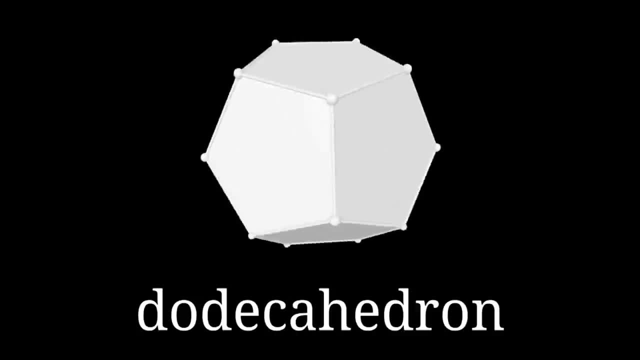 put three pentagons around a vertex and eventually you get the 12-sided dodecahedron, and any more than that is once again too many to fit around a vertex. you could start with hexagons, but three hexagons is already too many, so we've reached the limit, and so we can convince ourselves that these 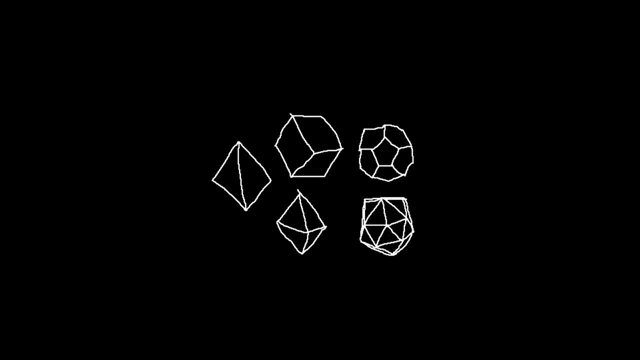 are the five regular polyhedra and you might look at that and say, yeah, that makes sense. I mean, what else could you do to make another one? the faces have to be regular polygons and those are the only three polygons where you can fit three around a vertex, and you've exhausted all the 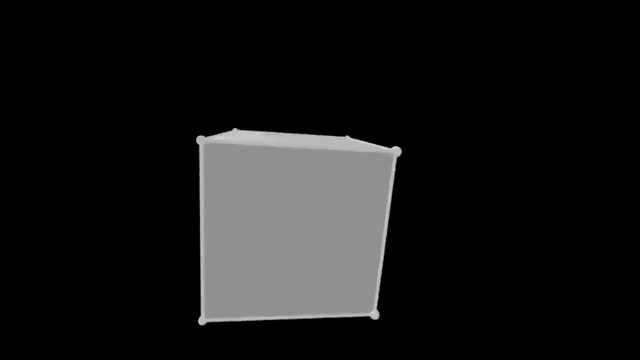 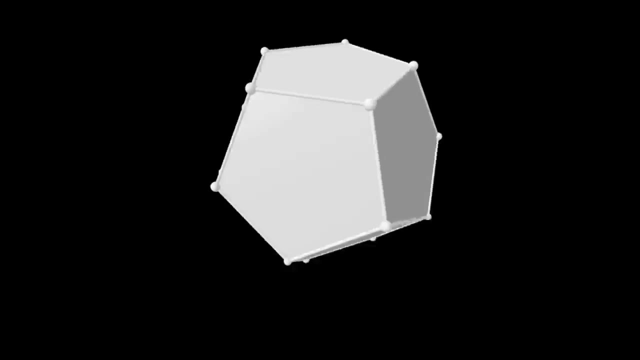 of each. you can put around a vertex and, yeah, using these three polygons as faces. these are the only five closed convex 3D shapes we can construct that fit the definition of a regular polyhedron. but is there any reason to assume that these are the only three regular polygons? you? 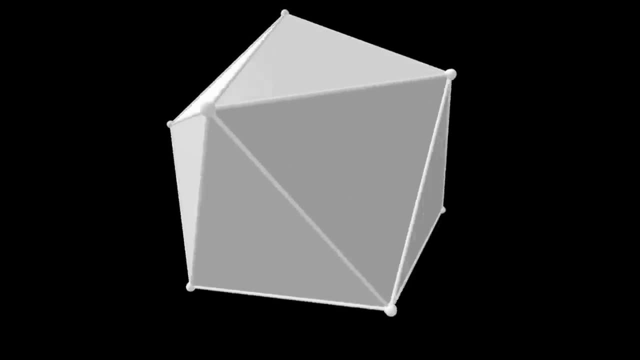 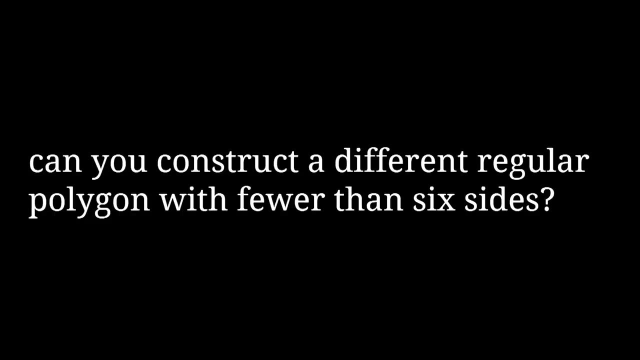 could use as faces. now you might be thinking: well, yeah, of course everything with more sides than a pentagon won't fit, and you're right about that too. but what if you could construct a different regular polygon with fewer than six sides? could that work? the answer: surprisingly. 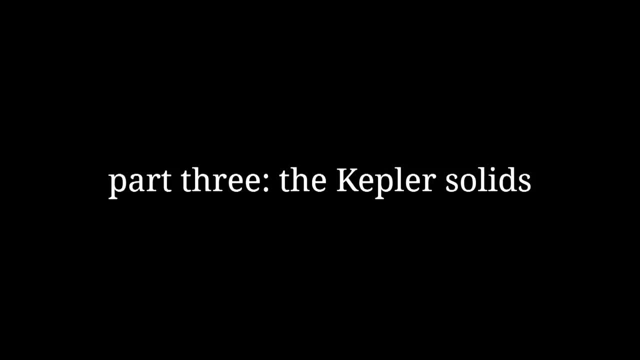 is yes. let's get back down to 2D and look at regular polygons. if you have at least three line segments that are all the same length, you can use them to construct a regular polygon. so if you have five line segments, you can arrange them like this and make a regular pentagon. but 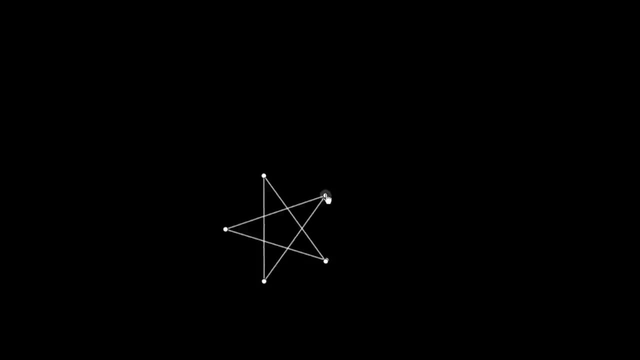 what if you did something like this? this is a pentagram, also known as a five-pointed star, and it's a perfectly good regular polygon. you might say that can't be a regular polygon. see, that vertex isn't the same as that vertex, so it isn't vertex transitive. this is cheating, but the 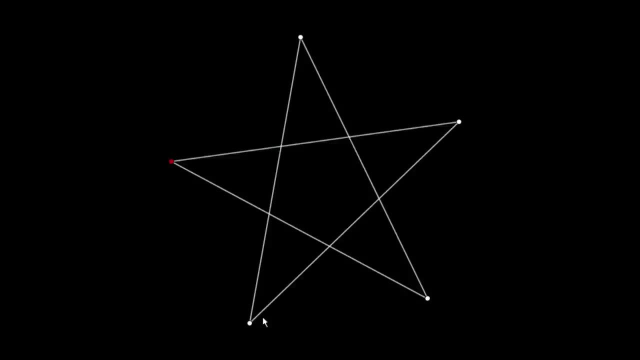 point is, those self-intersection points aren't vertices. this polygon has five edges and five vertices, just like a regular pentagon, and it has the same exact amount of symmetry as a regular pentagon. true, it's not convex and it does intersect itself, but there's nothing in the 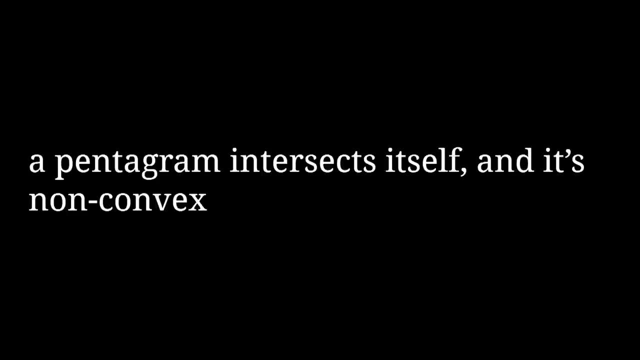 rulebook that says a golden retriever can't construct a self-intersecting, non-convex regular polygon. unless we amend our definition to explicitly exclude shapes like this, it must be included. the pentagram is part of an infinite family of star polygons. 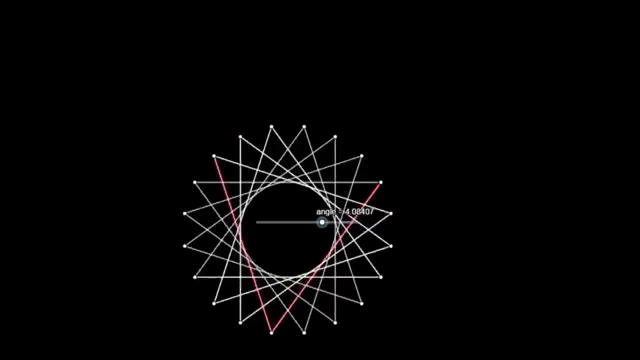 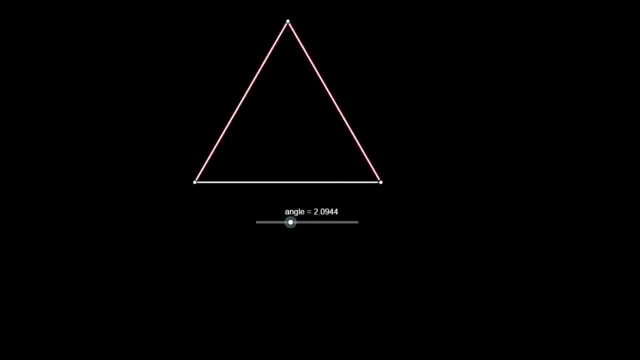 taking them into account, we can say that there is one regular polygon corresponding every rational angle. that means that if you start with two line segments and have them meet at some angle which can be described as some fraction of a circle, you can connect their 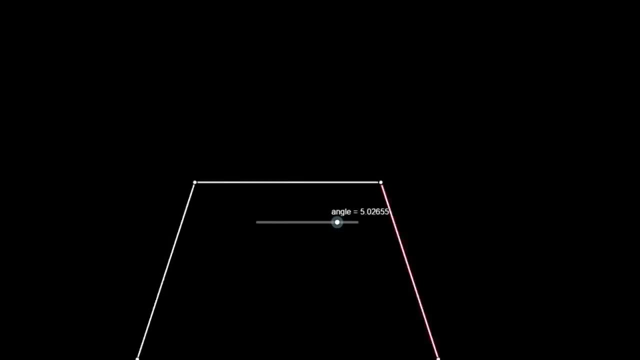 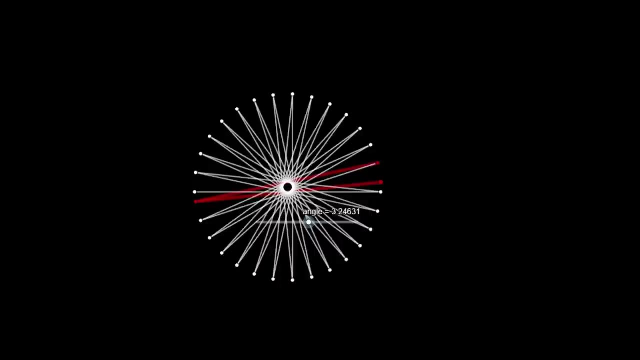 disconnected ends with similar line segments that meet at the same angle and eventually, by continuing to do that, you'll get some closed shape which fits the definition of a regular polygon. I think that's pretty cool, while there are indeed infinitely many regular star polygons. 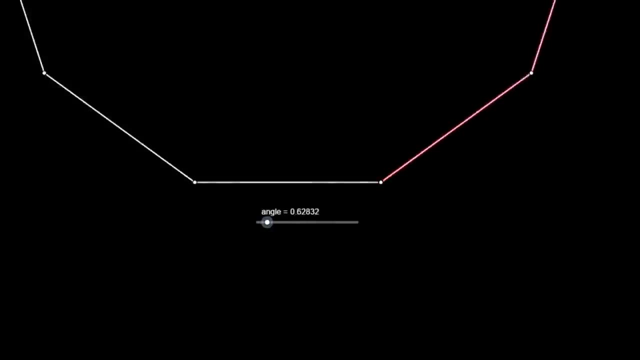 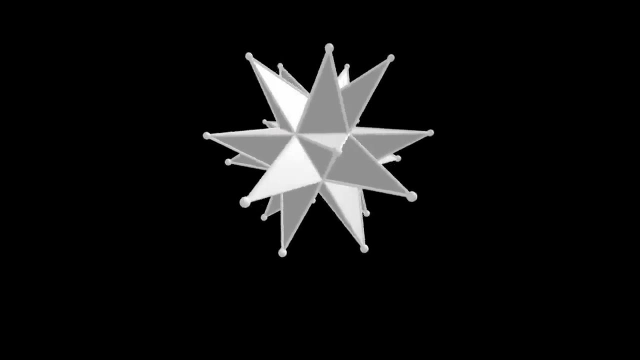 the only one that will work as the face of a regular polyhedron is the pentagram. so let's try it out. put three pentagrams around a vertex and what you eventually get is this really cool looking shape, and I mean, just look at it. what even is this spiky thing it's made out of? 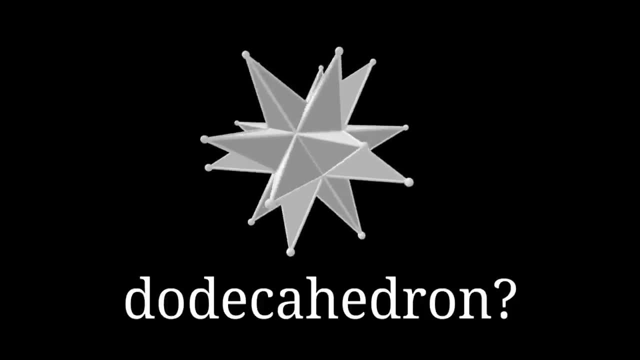 12 pentagrams, so it's a type of dodecahedron. since it's a star, you could call it a stellated dodecahedron. let's see what else you can do with pentagrams: five pentagrams around a vertex ends. 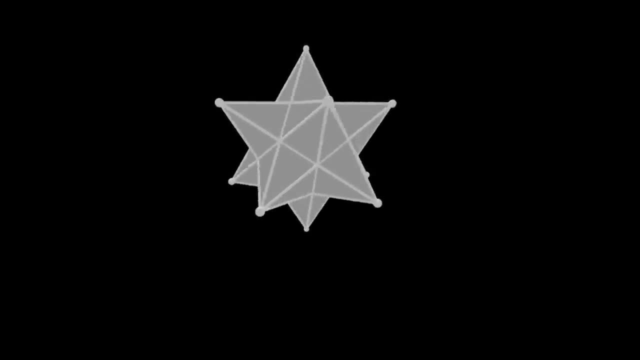 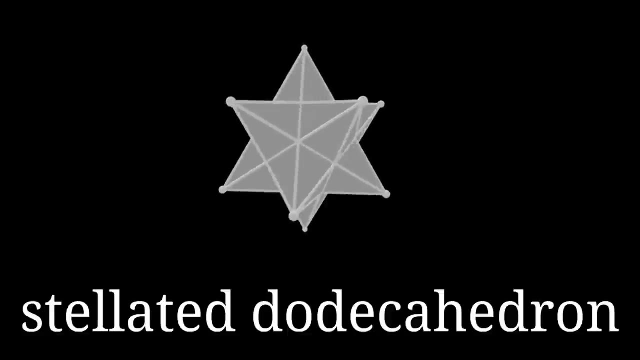 up forming another closed shape. unlike the stellated dodecahedron we made earlier, which had 12 pentagramal faces, this one has 12 pentagramal faces, so I guess this one is also a stellated dodecahedron. okay, since this one isn't as spiky as the other one, let's call. 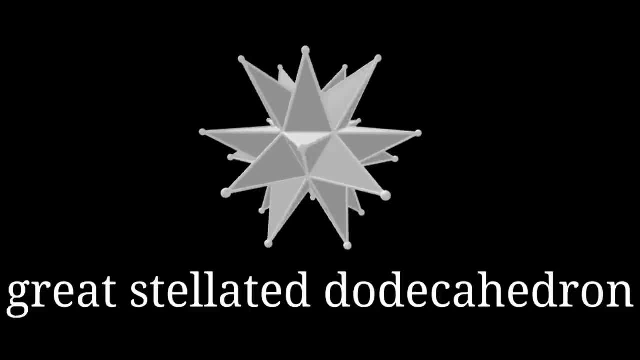 it the small stellated dodecahedron, and we'll call the other one the great stellated dodecahedron. another way of thinking about the stellated dodecahedron is by starting with a dodecahedron. 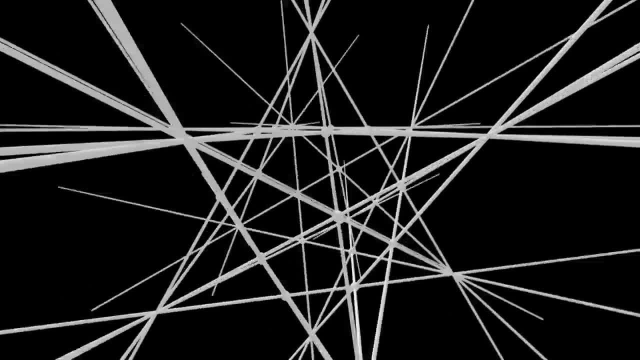 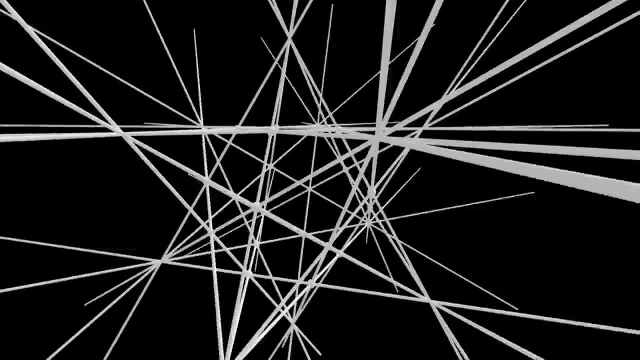 and then making its edges longer until they meet up on themselves again. this process is called stellation. this pair of regular star polyhedra was described by Johannes Kepler in 1619, so they're called the Kepler solids as companions to the platonic solids. and so we can now conclude. 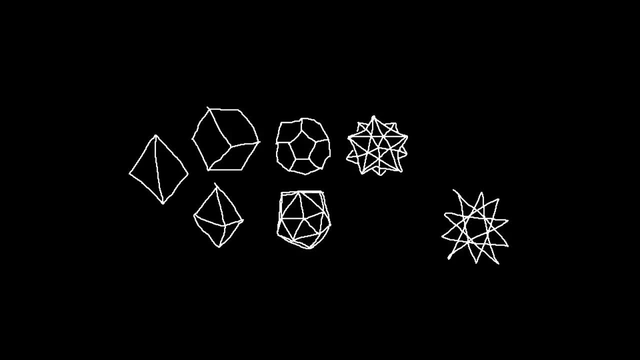 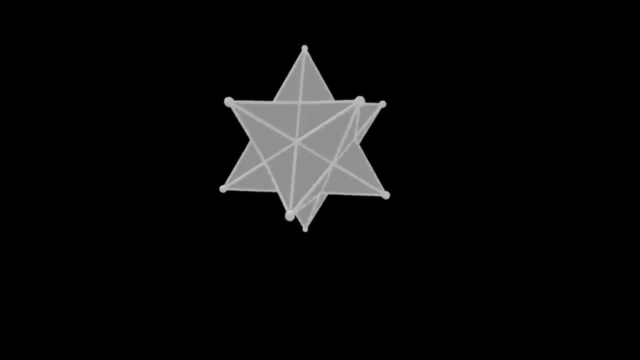 that there are seven regular polyhedra, except we're still not done with star polyhedra. almost 200 years after Kepler described the Kepler solids, a mathematician named Louis Poinceau found another pair of regular star polyhedra, which later were shown to complete the set. 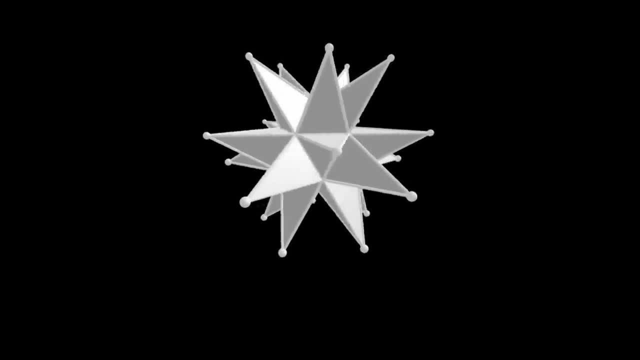 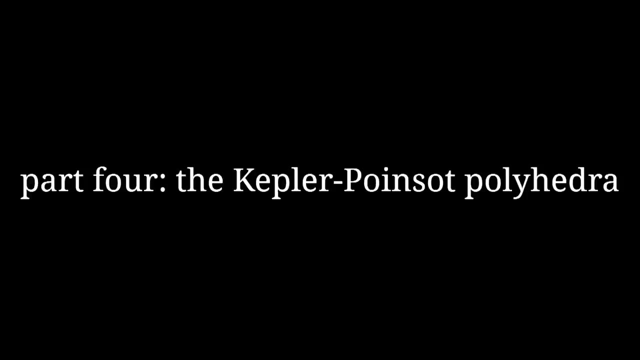 today the four regular star polyhedra together are called the Kepler-Poinceau polyhedra. part four, the Kepler-Poinceau polyhedra. to describe what Poinceau found, we'll first need to get back to the idea of a Schlafly symbol. as I showed before, a Schlafly symbol defines each 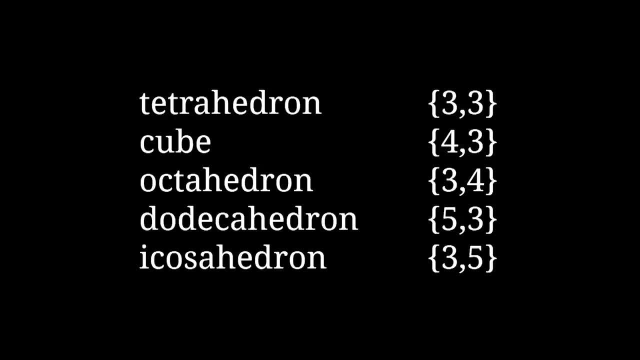 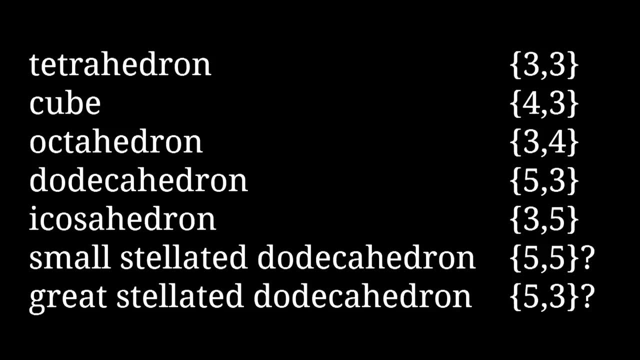 regular polyhedron as the number of edges of each of its faces, followed by how many faces meet together at each vertex. while this definition works for the platonic solids, it doesn't work for the star polyhedra, since a pentagon and a pentagram have the same number of sides: the 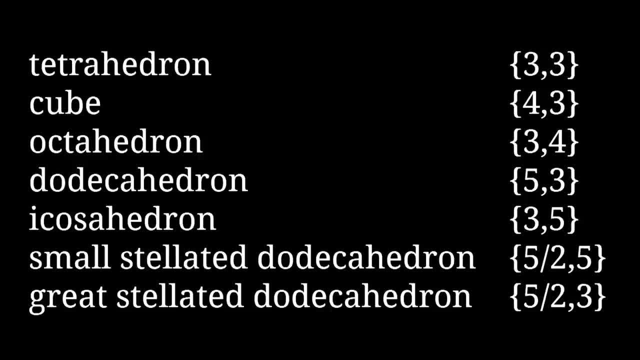 reason for this is to represent pentagrammal faces with the number 5 over 2 instead of 5.. there is a reason for this which I will not be explaining, so just trust me that this makes sense and isn't just arbitrary notation. so the small and great stellated dodecahedron have the symbols. 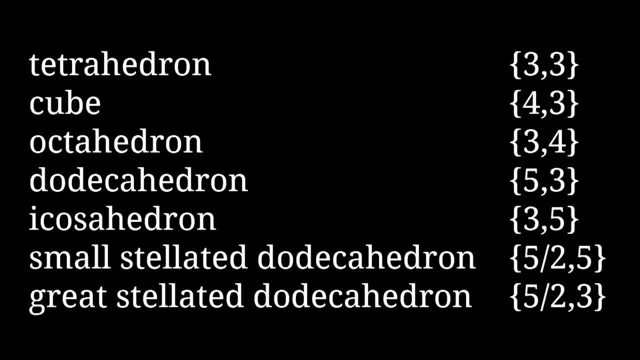 5 over 2, 5, and 5 over 2, 3, respectively. now, the fact that star faces are represented in this way means that the first number doesn't really mean the number of sides of each face, it's just. 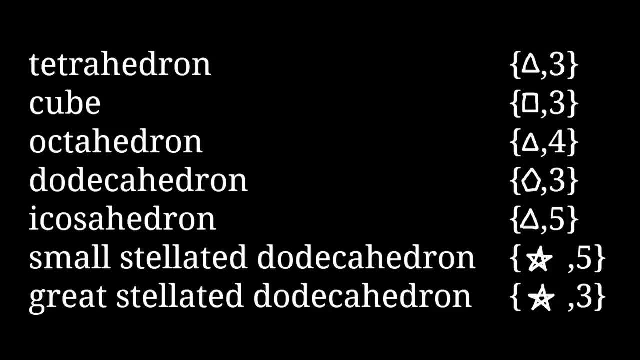 a number that's used as the name for a specific regular polygon. so then, what about the second number in the symbol? are the numbers actual numbers or are they notational shorthand for specific polygons? the answer is the latter. take the symbol for a cube: 4, 3.. this can be understood to mean square triangle, but what about a cube? 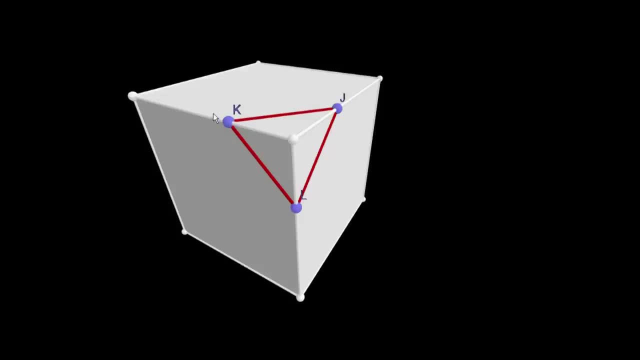 is triangular. well, if you look at one vertex where three square faces meet, you can slice through a cross section and you'll see a triangle. you can say that a cube's vertex figure is a triangle. oh and, by the way, this Wikipedia animation I'm using here is showing how 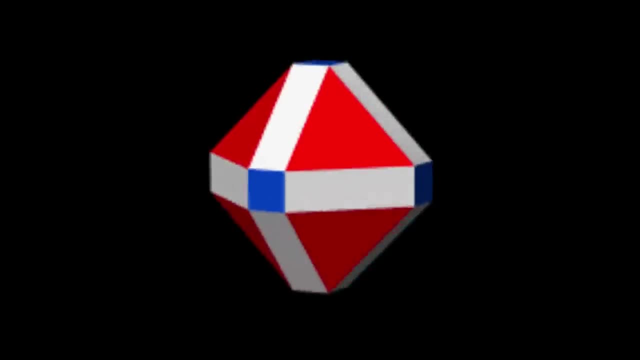 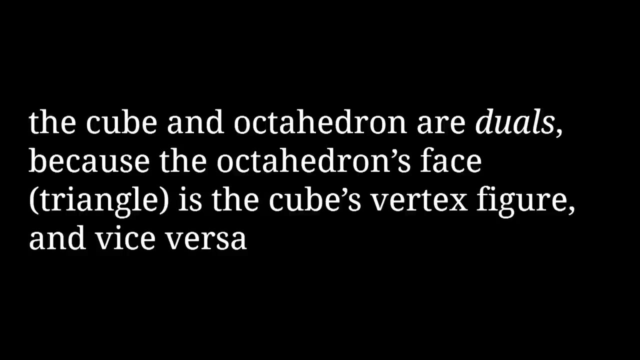 if you slice through all the faces of a cube at once, you get an octahedron. an octahedron is the square faces and triangular vertex figures, and an octahedron has triangular faces and square vertex figures. so who cares? why does any of this matter? well, just like how a face doesn't. 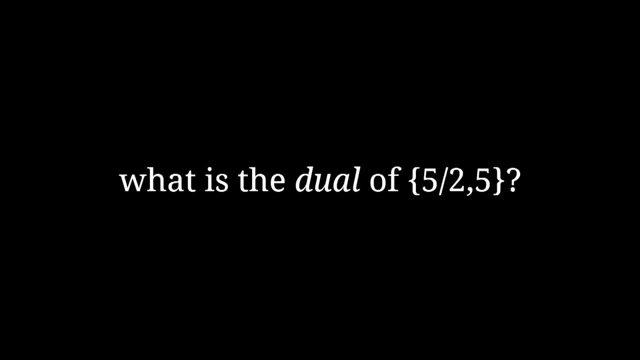 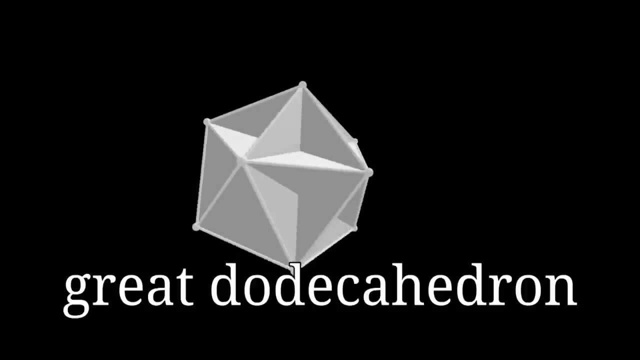 have to be a convex polygon. a vertex figure doesn't have to be a convex polygon either, and that's what Poinsot found. if you make a shape with pentagons as its faces and pentagrams as its vertex figure, you get a great dodecahedron. and doing the same thing with triangles gets you 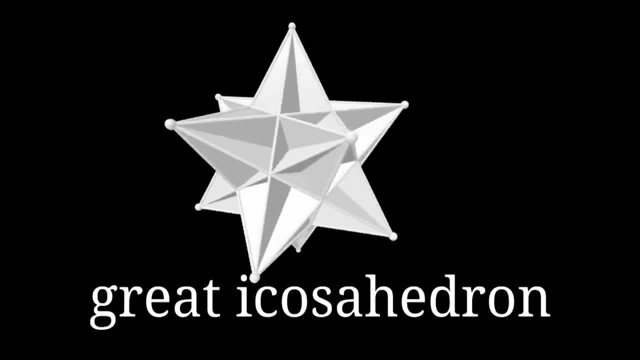 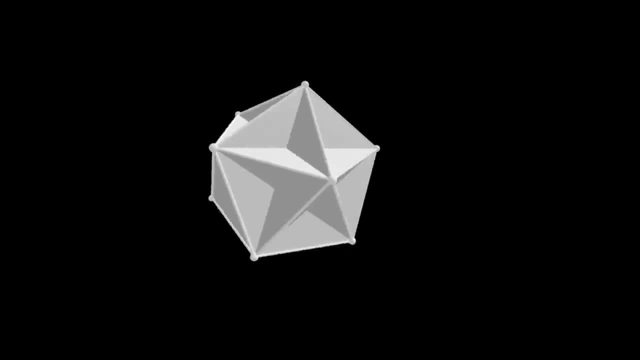 a great icosahedron, and if you try it with squares, it just doesn't work. another way of thinking about the Poinsot polyhedra is to think of taking a dodecahedron and an icosahedron and making their faces larger rather than making their edges longer. this 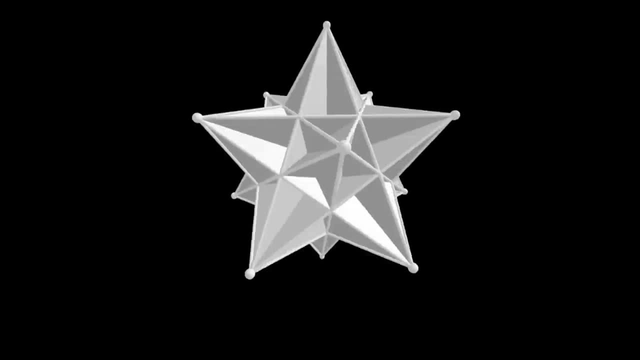 is another type of stellation called gratenning. anyway, together with the pair of stellated dodecahedra, we now have all four Kepler-Poinsot polyhedra and if grouped in with the platonic solids, we can now say that there are nine regular polyhedra. I really like the Kepler-Poinsot. 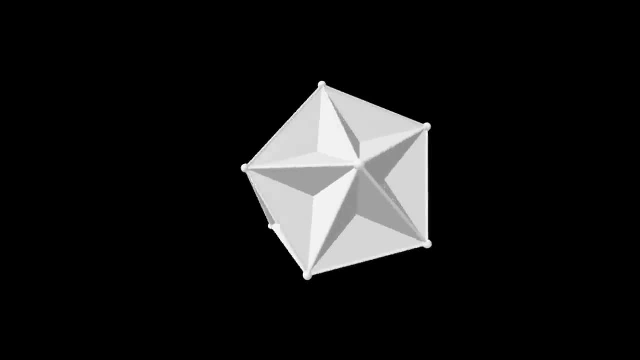 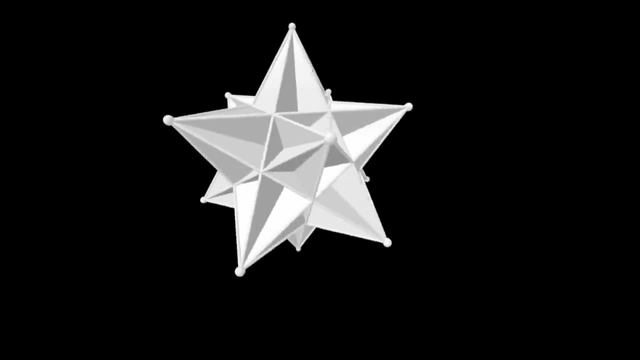 polyhedra. they have most of the same properties as the platonic solids, except that they objectively look way cooler because of all the spikes. they're super underrated and I think more people should know that they exist. the rest of the regular polyhedra: 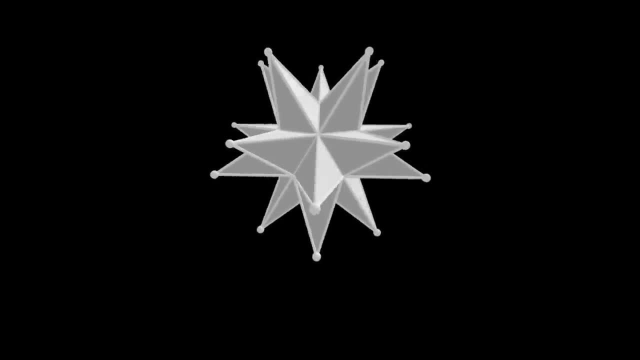 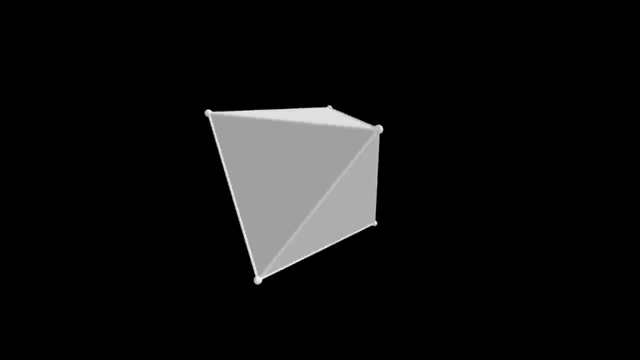 all fit the definition, but they're not what you'd call solids. you'll see what I mean. part five: the regular tilings. what we've seen so far is that you can use triangular faces to make tetrahedra, octahedra, icosahedra and great icosahedra. you can use square faces. 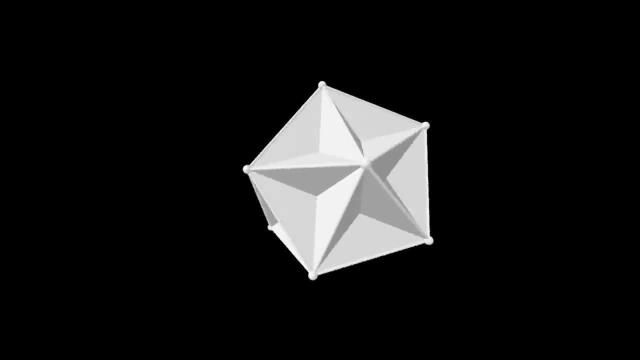 to make cubes. pentagonal faces to make dodecahedra and great dodecahedra and pentagrammal faces to make small and great stellated dodecahedra. hexagonal faces just don't work, but like: 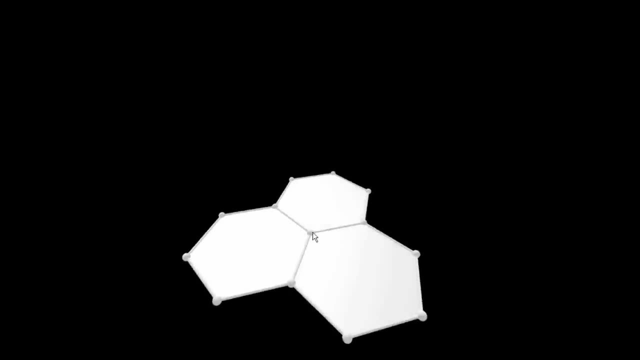 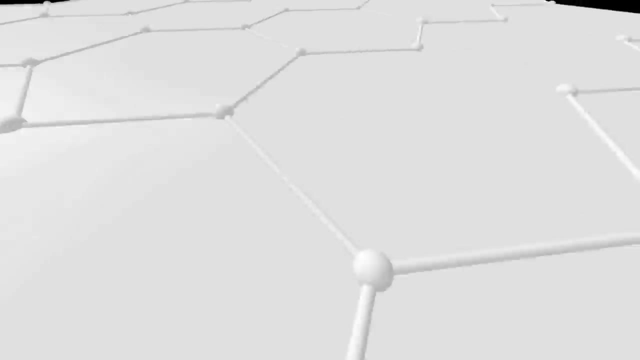 why not? you can fit three of them around a vertex just fine. it's not like heptagons, where they don't fit at all. in fact, if you keep going, you eventually get something like this: a polyhedron with infinitely many hexagonal faces. it has a few names. 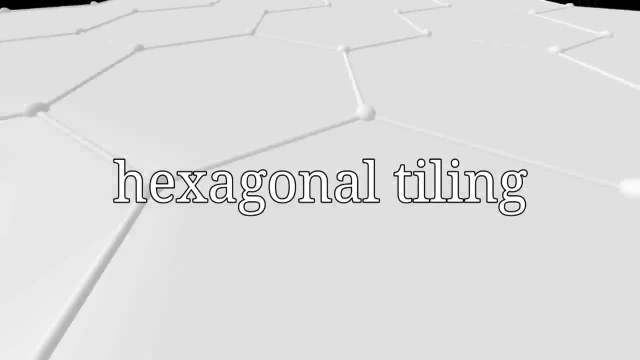 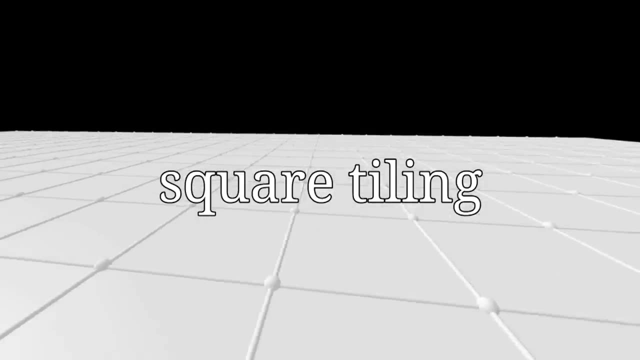 but it's most well known as the hexagonal tiling. it's one of three regular tilings of the plane, along with the triangular tiling and the square tiling. true, these are not closed shapes like the platonic solids and the Kepler-Poinceau polyhedra, but they still fit the definition. 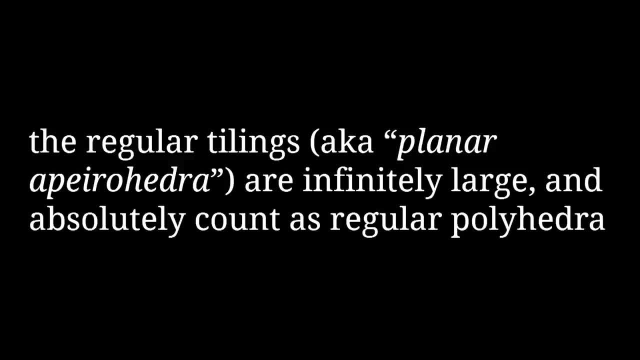 of regular polyhedron. you can move any face to any other face, any edge to any other edge or any vertex to any other vertex. they're flat, they're infinitely large and they're regular apirahedra. once again, even if you feel like they shouldn't be in the same category as the. 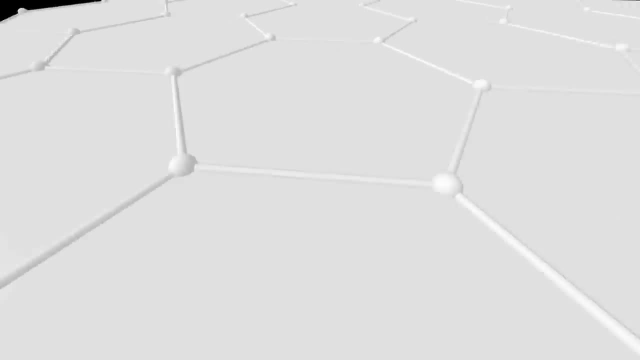 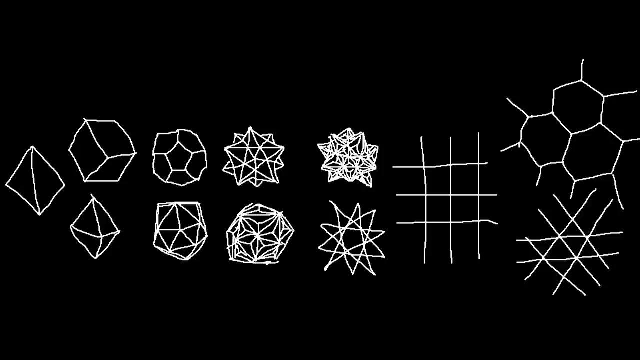 other regular polyhedra. you'd need to specifically change the definition of regular polyhedron to exclude them. just because they're infinitely large doesn't mean they aren't allowed, and so finally, we have all 12 regular polyhedra. and really, when I first started this video, 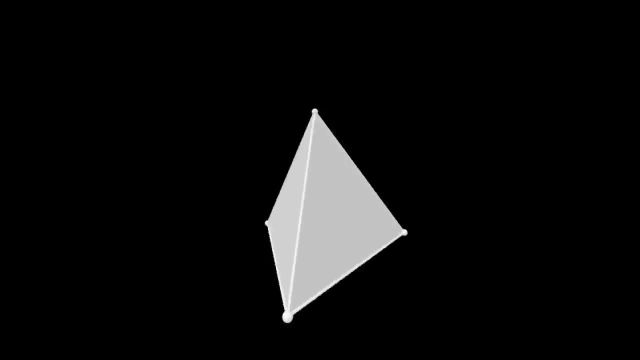 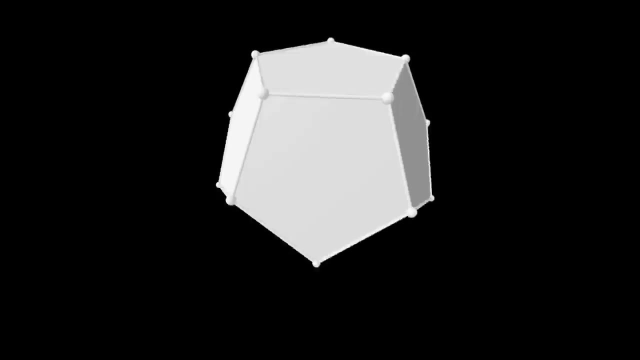 I was going to leave it at that. I was going to make a video called there are 12 regular polyhedra, where I talked about how often the Kepler-Poinceau polyhedra and the regular tilings are left out of discussions about regular polyhedra, even though they're just. 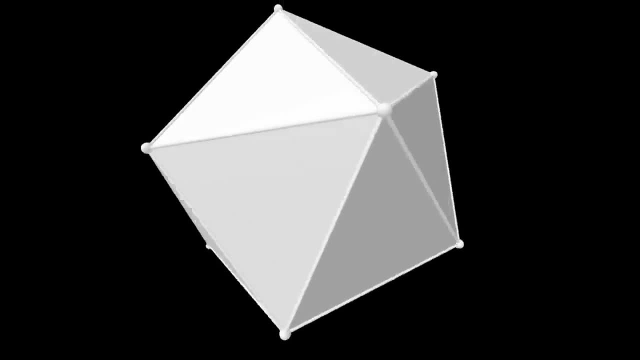 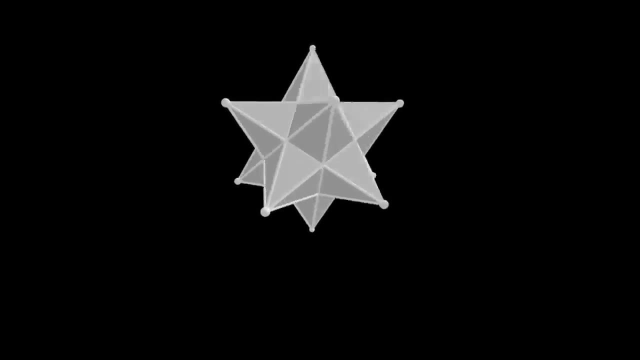 as cool as, if not cooler than, the platonic solids. it would have been fun. you know, I could have gone into things like what sorts of new shapes are allowed when you remove some of the restrictions. I could have had a reason to bring up the stella octangula, but as I was doing the 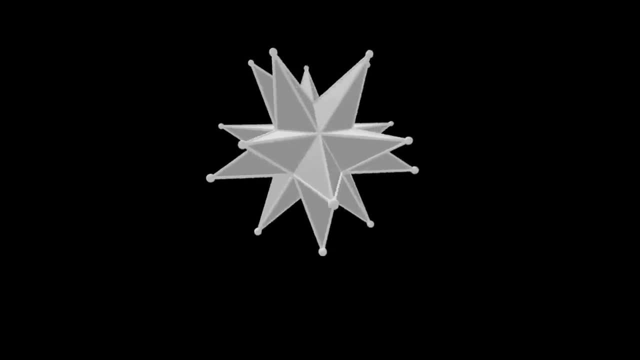 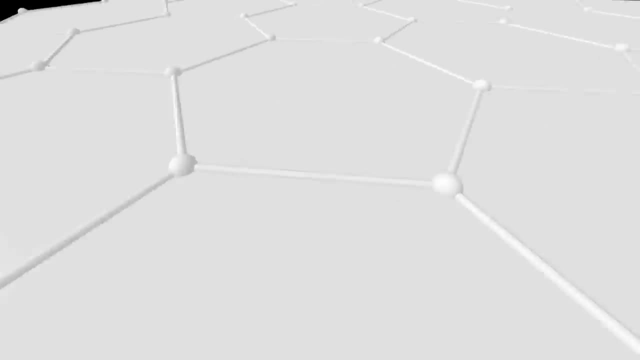 bare minimum amount of research necessary to make sure I wasn't missing any regular polyhedra, I found something. it turns out I was missing some. I was missing quite a few, in fact so many that it would have been very silly to put out a video saying that there's exactly 12 of them. 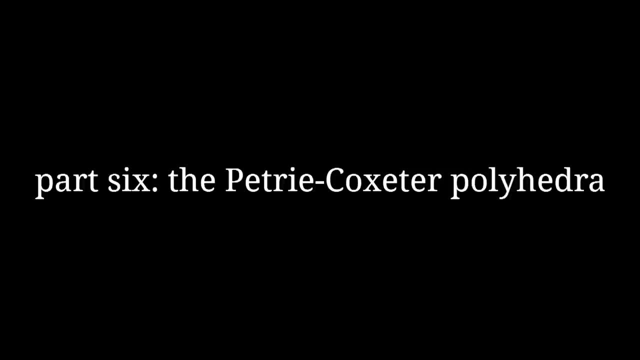 part six: the petri-coxeter polyhedra. in 1926, John Petrie discovered a pair of infinite polyhedra which, unlike the regular tilings, are not flat. shortly afterwards, Petrie's fellow geometer, Donald Coxeter, found a third one. 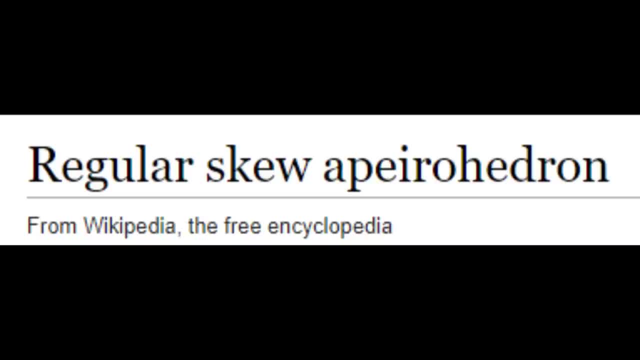 Wikipedia calls these the regular skew epirohedra, but I think calling them the petri-coxeter polyhedra is more fitting. before I can explain the petri-coxeter polyhedra, it'll be helpful to start with an analogy in polygons. imagine a triangle now. 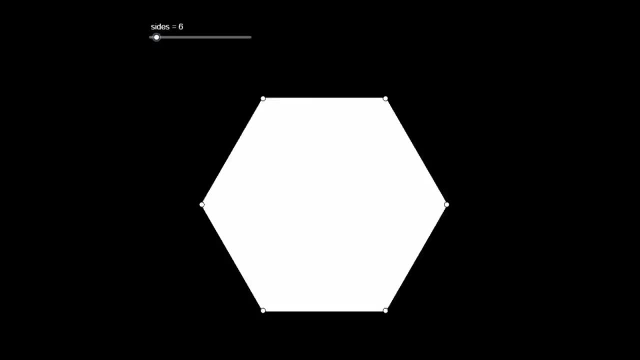 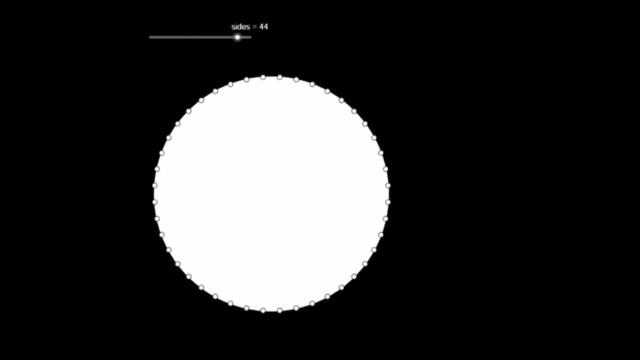 add one side and make it a square, add another side and make it a pentagon, and keep doing that. as you keep adding more sides, the shape you get starts looking more like a circle and once you have infinitely many sides, you end up with an epiragon which looks exactly. 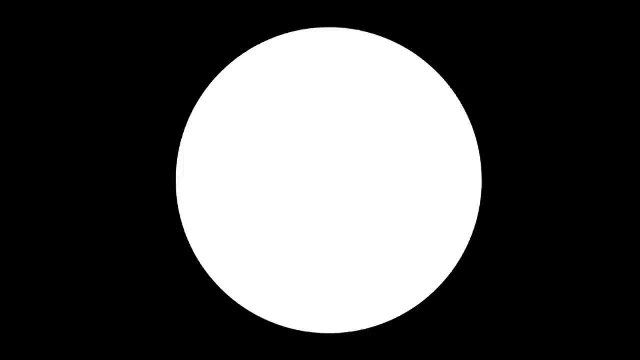 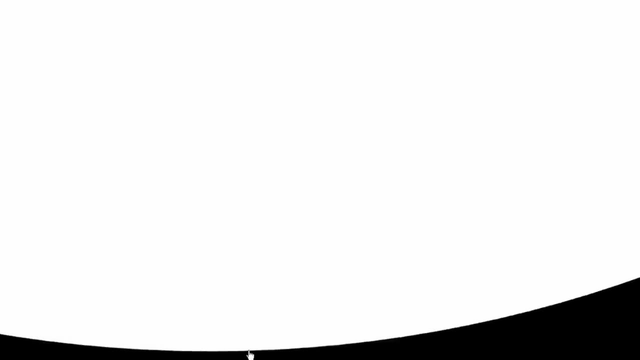 like a circle, but it only looks like a circle because we're too far zoomed out to see the individual edges. indeed, since there are infinitely many of them and since the circle has a finite circumference, if we're thinking about the regular epiragon as being like a circle, 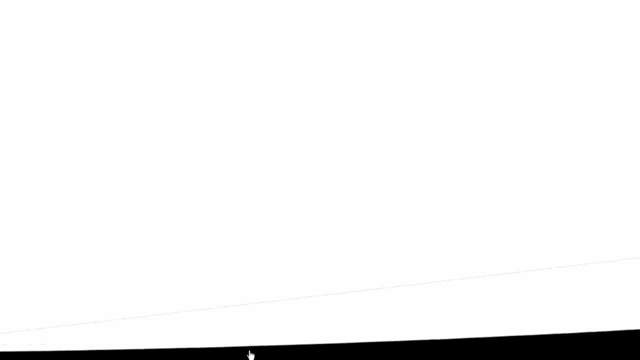 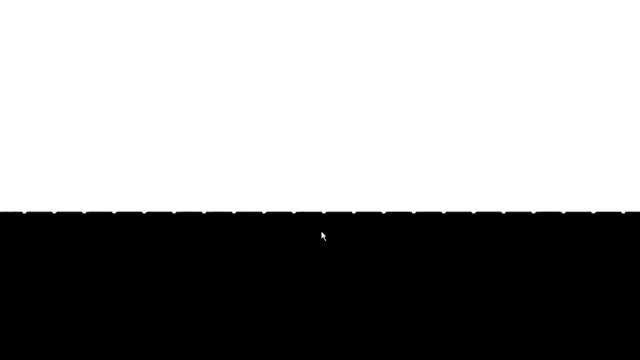 each edge must be infinitesimally small. so let's zoom in infinitely far so we can see the individual edges. at this zoom level it doesn't look like a circle at all. it looks like a line, just like the regular tilings of the plane. this is an infinitely large shape. that's. 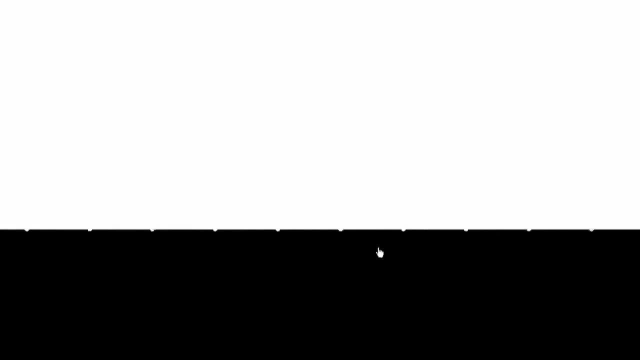 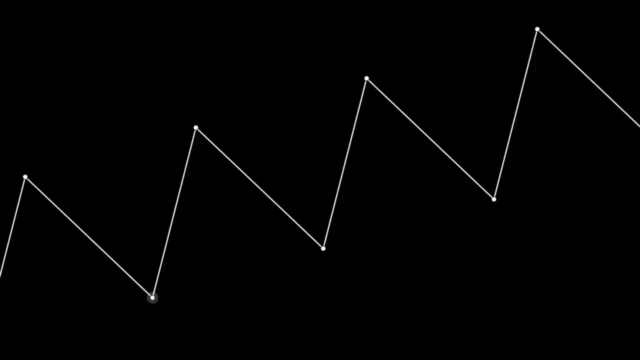 also completely flat. can you make a regular epiragon that isn't flat? well, yes, you can. all you need to do is something like this: this is a shape which infinitely alternates between its edges, going up and down in a regular pattern. the technical name for this shape is a zigzag. 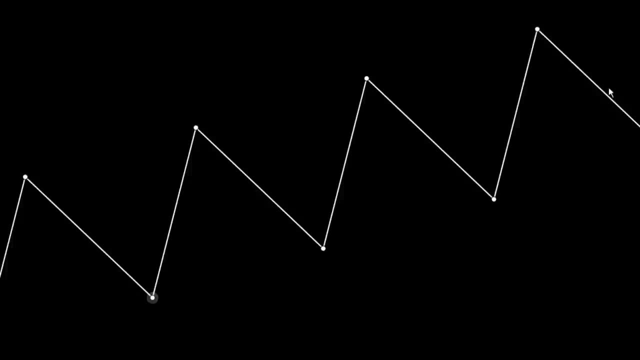 and a zigzag is entirely within our definition of a regular polygon. it doesn't actually matter what the angle is, so a zigzag can be however wide or narrow you want. the key observation that leads from zigzags to the petri-coxeter polyhedra is this: look closely at this square. 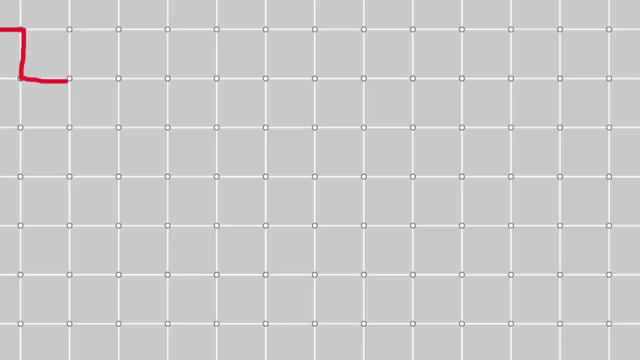 tiling. you can see here that within this grid there exists a clear zigzag pattern, and in fact the same thing can be found in the other two regular tilings. maybe by examining tilings of 3d space, we'll be able to find infinite polyhedra that aren't flat, and that's exactly what petri and 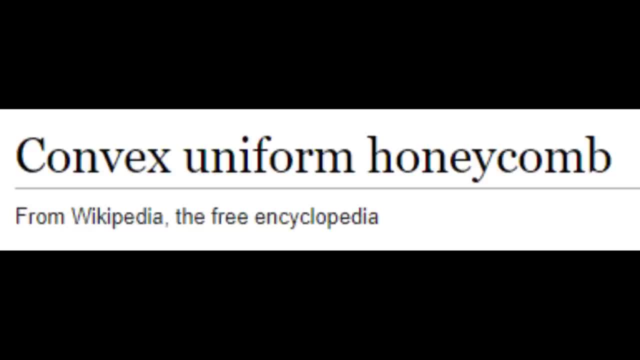 coxeter did. tilings of 3d space are usually called honeycombs, which i think is specifically to make it so you can't call the hexagonal tiling a honeycomb, tiling all three of the petri-coxeter. 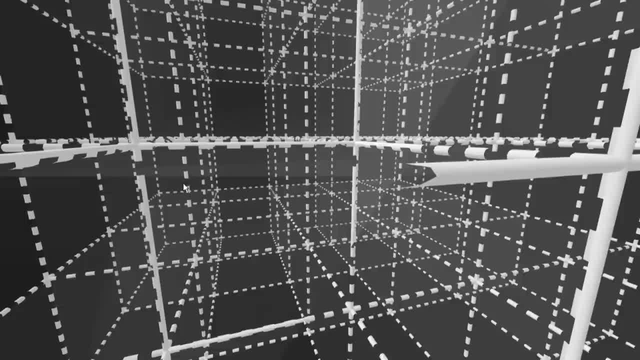 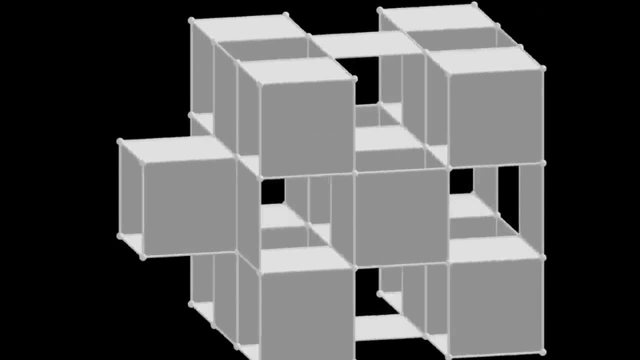 polyhedra are derived from the cubic honeycomb. the cubic honeycomb is a tiling of 3d space made out of many cubes. by following a zigzag-like pattern along the square faces of all the cubic cells, you can end up with a regular polyhedron called a mu-cube- a helpful way to think about the mu-cube. 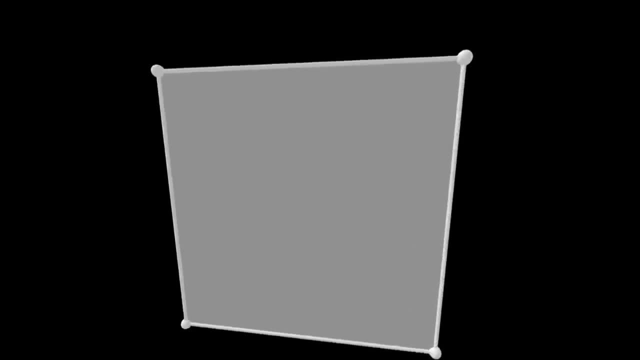 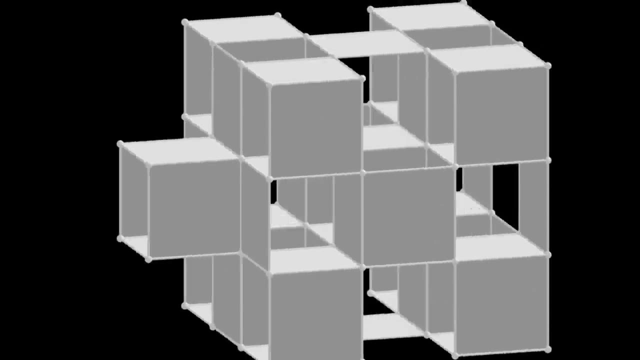 is to think of it as being made out of cubes that have two opposite faces missing. by arranging six of these almost-cubes in a cube-like form, you get the basic building block of the mu-cube. this can be extended infinitely to get the real thing. next is the mu-octahedron, which is based on. 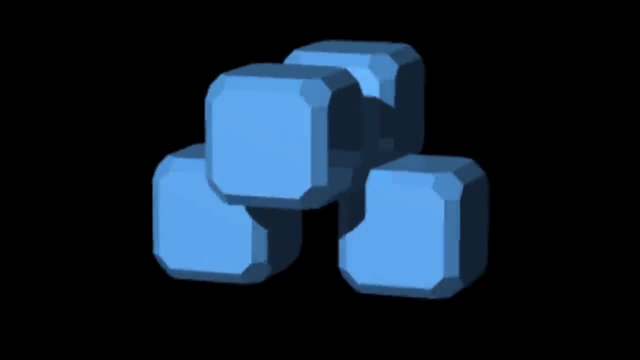 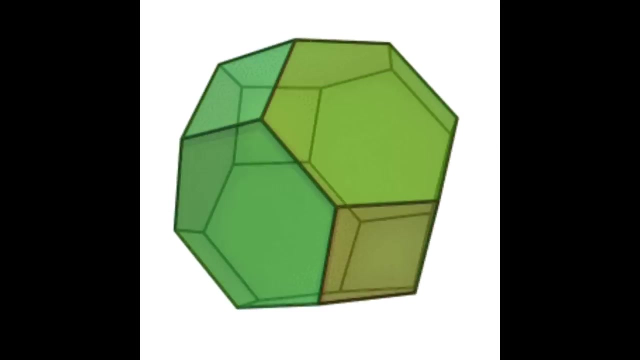 a bitruncated cubic honeycomb. while this honeycomb is derived from the cubic honeycomb, it'll be easier to explain how it's structured from the ground up. its cells are not cubes, but rather truncated. octahedra truncation is this process that i like to think of as being like cutting off? 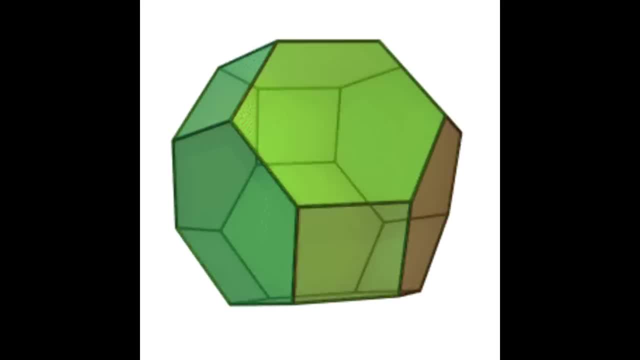 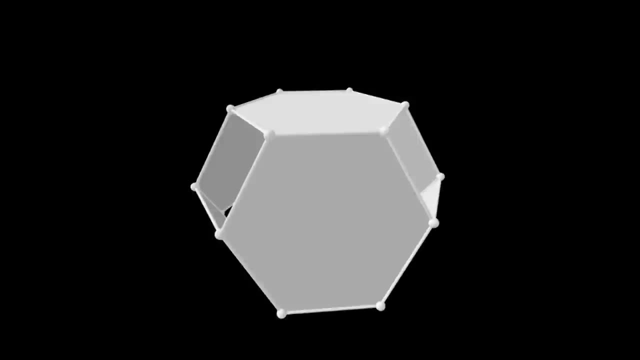 the corners of a polyhedron. when you truncate an octahedron, its eight triangular faces become hexagons and its six vertices become squares. this shape isn't regular because it has two different types of faces, but it can be used to tile 3d space and by simply removing all 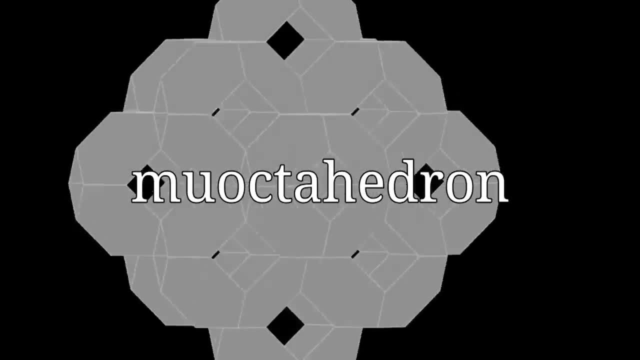 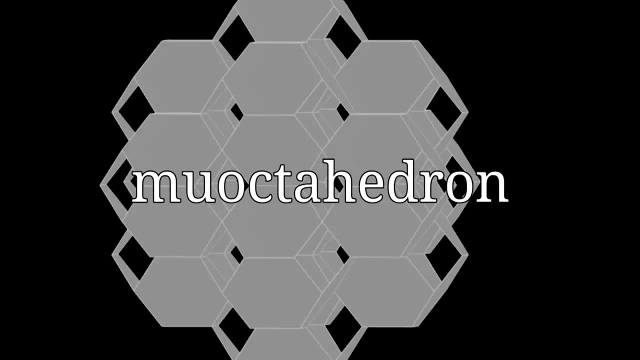 the squares. from this tiling you get another regular polyhedron. the third petri-coxeter polyhedron, which was coxer's contribution, is the mu-tetrahedron. it's based on the quarter-cubic honeycomb. it's derived from the cubic honeycomb, but it'll be. 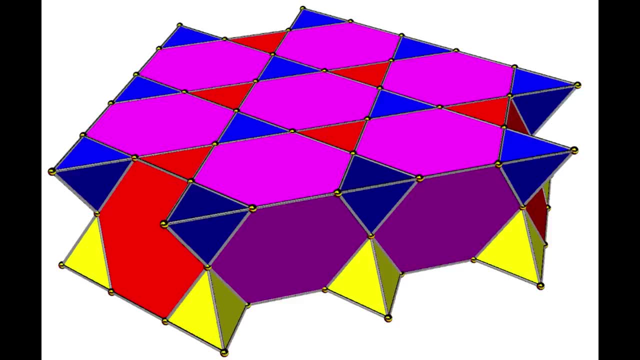 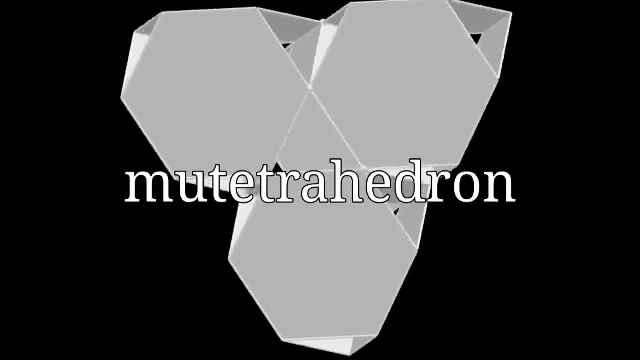 easier to explain its structure if we talk about its cells instead. the cells of the quarter-cubic honeycomb are tetrahedra and truncated tetrahedra. by removing all of the triangular faces of a quarter-cubic honeycomb, you end up with a mu-tetrahedron, and so there we have it, three. 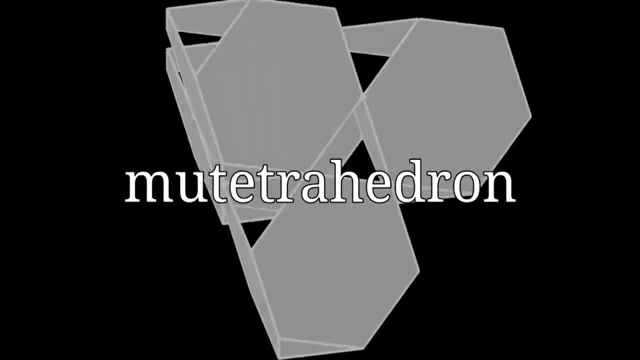 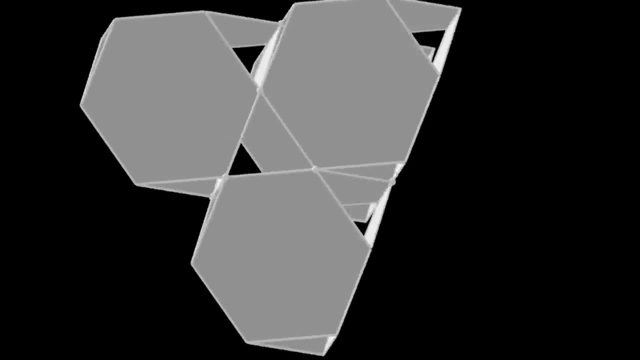 completely regular infinite polyhedra and, unlike the regular tilings, these babies have some actual depth to them. you've got the mu-cube made out of infinitely many squares, and the mu-octahedron and mu-tetrahedron both made out of infinitely many hexagons. this is exciting stuff, taking these, 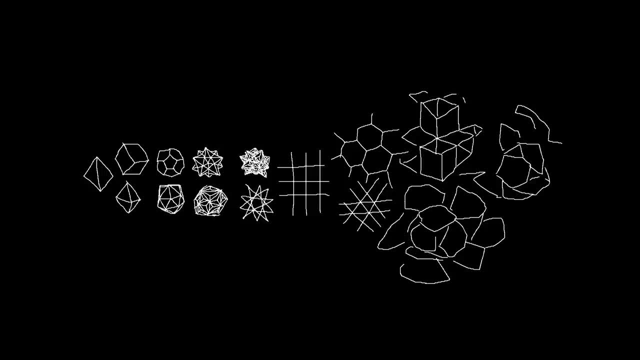 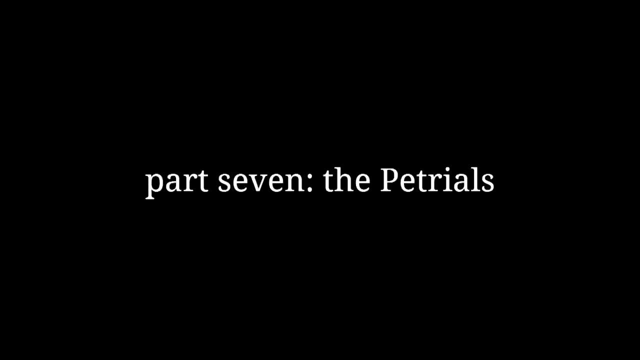 into account, we can now say that there are, in fact, 15 regular polyhedra. from here, things are going to get a lot weirder. part seven: the petrials. what exactly is a polygon? yeah, I defined it earlier, but there might still be some assumptions that you're making that weren't. 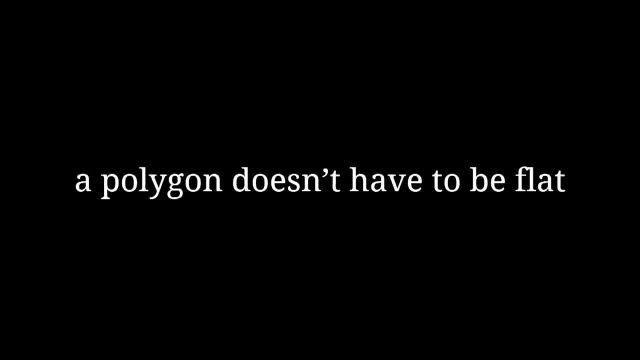 a part of it. for example, there is nothing in the definition that restricts polygons to two dimensions. let's say you were to take a zigzag, but rather than it just going off infinitely, you fold it up into the third dimension and you have it meet back on itself. this has some rather 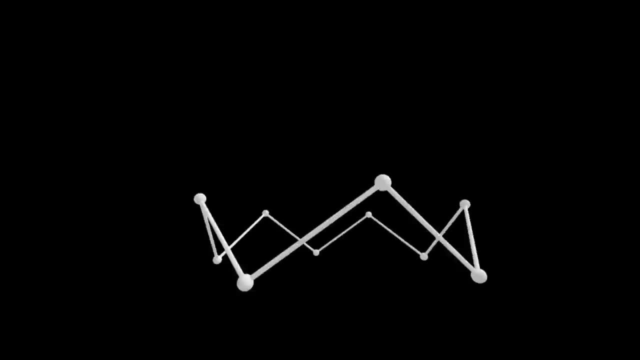 big implications like: okay, what is the area of this polygon? see, the question doesn't even make sense anymore. this thing doesn't have area. it doesn't even have an inside. this is what's called a skew polygon, and they're huge game changers. so what do you get when you try to? 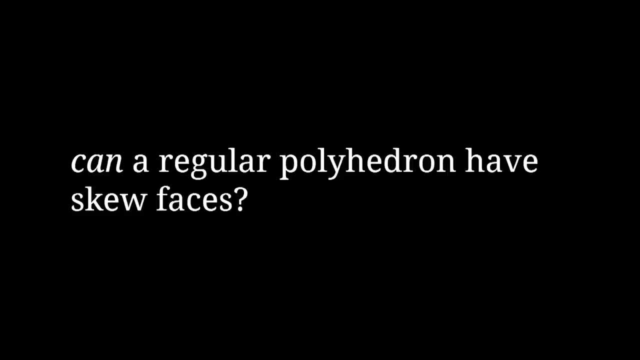 make a polyhedron with skew polygons as its faces. this sounds tricky, just like zigzags. it's not necessary for them to have set rigid structures to be regular. you can move them about and deform them while preserving the defining symmetries. where would you even begin? 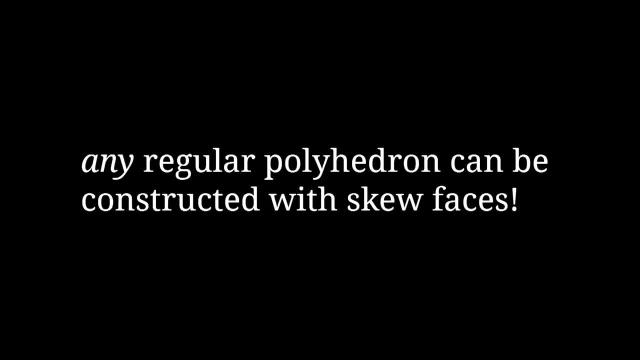 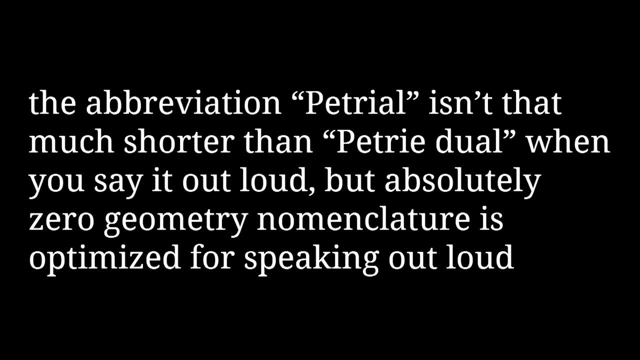 what petri found was that you can actually take any polyhedron made out of normal flat polygons faces and convert it into another polyhedron made out of skew polygon faces. this is called the petridule or petrile of the polyhedron. take the cube, for instance. let's rotate this. 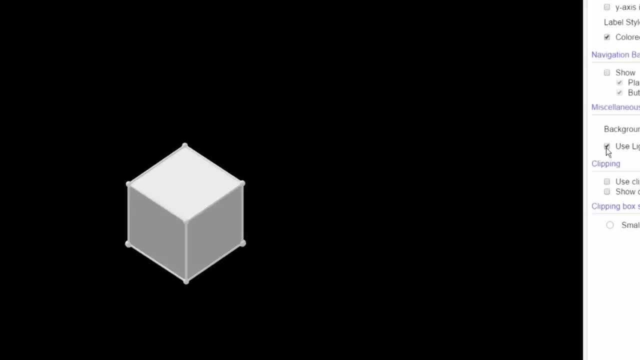 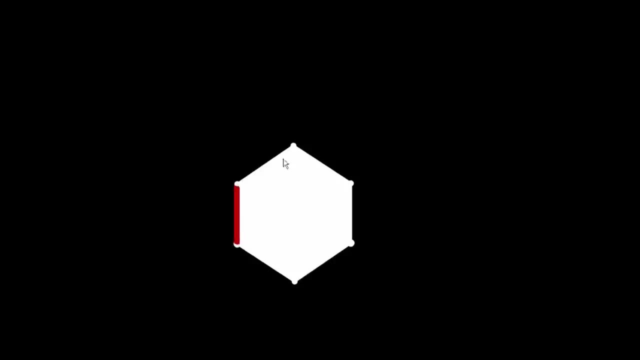 cube, so we're viewing it with one vertex facing us. now look at the cube's silhouette. it sure looks a whole lot like a regular hexagon, doesn't it like? maybe you could trace along this edge and draw a hexagon- along the edges of this cube, of course, once you rotate it again. 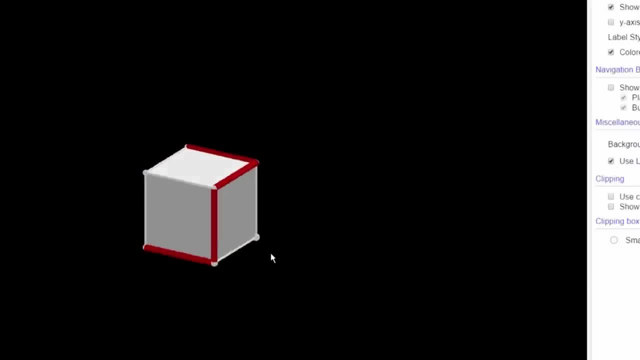 the illusion breaks and it doesn't look like a regular hexagon anymore. but it is a regular hexagon. this is a regular skew hexagon and it's built into the edges of a cube. this is called the cube's petri polygon. if you do this for half of the cube's eight vertices. 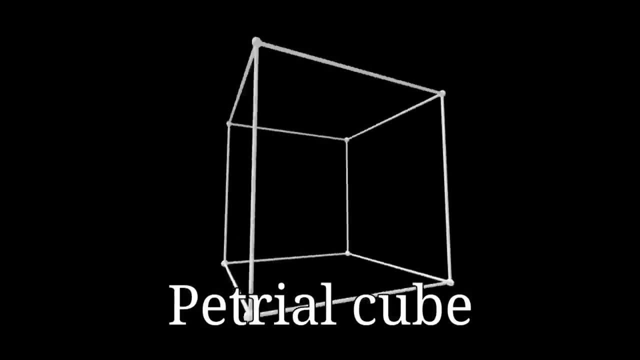 you can create a shape that looks exactly like a cube, but it's made out of four hexagons instead of six squares. sometimes finding the petri polygon of a regular polyhedron involves looking at its vertices, other times it involves looking at its faces, and sometimes you just gotta use the. 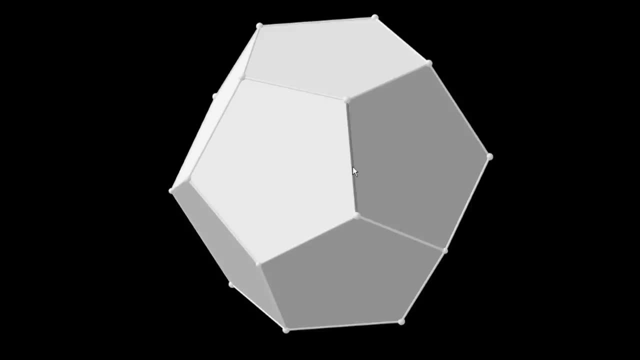 more formal definition, start at some vertex and follow along some edge that it's connected to. by definition, this edge will always be part of exactly two faces. you can continue along the line you've drawn, by turning left, so to speak, and following the face to the left of the edge. 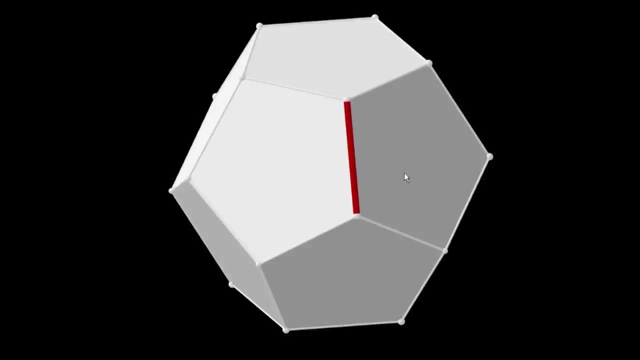 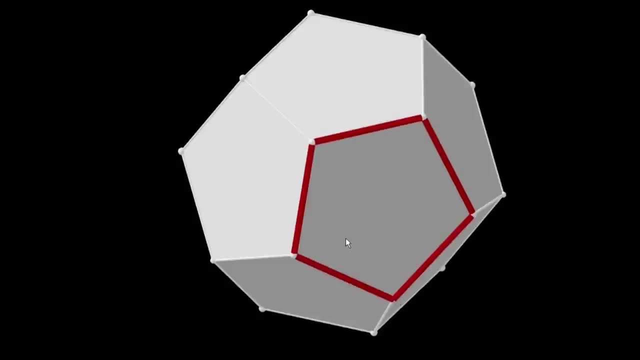 you've drawn, or you could turn right and follow along the face to the right. if you turn the same direction enough times in a row- in this case five, you will end up back where you started and you will have drawn one of the polyhedron's faces. but if, instead of doing that, you alternate, 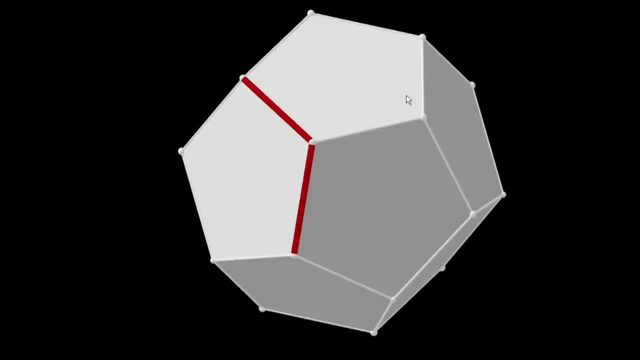 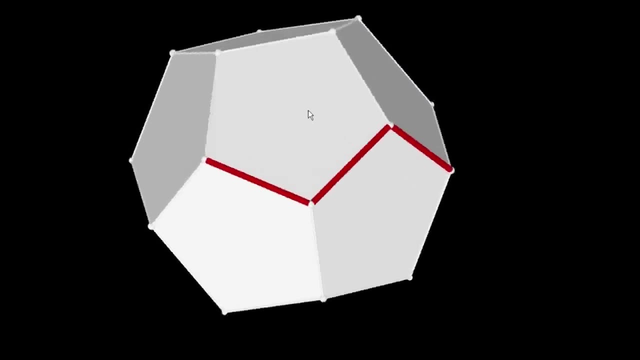 which way you turn each time, going left then right, then left then right, and so on. you will be tracing out the petri polygon instead. and, yeah, all 15 of the regular polyhedra we've gone over already have their own petrioles, giving us another 15 regular polyhedra you might be wondering. 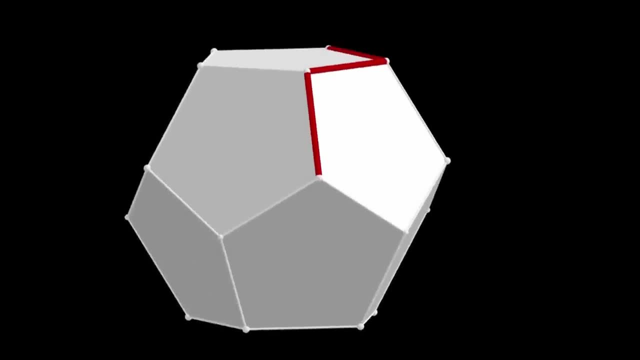 say: what if you find the petrioles of those petrioles? do you get another 15 new shapes? well, if you take, for example, the petriole cube and try to find its petriole, what you end up with? 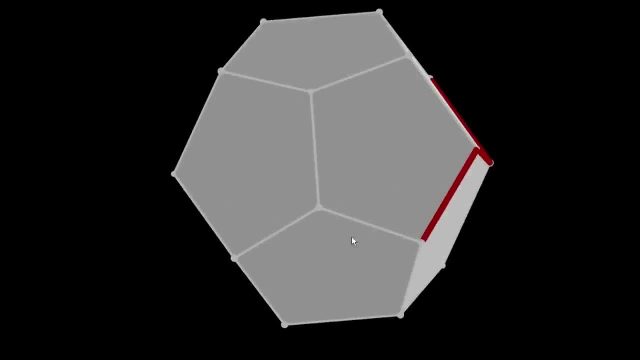 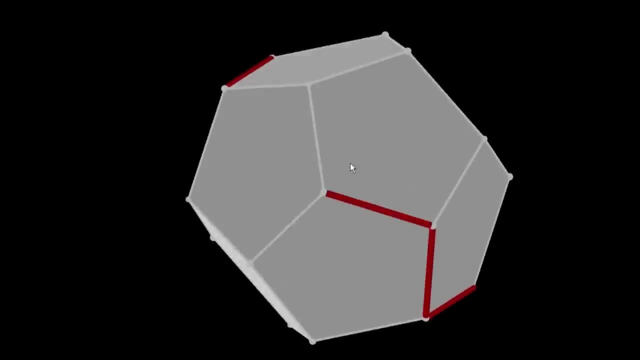 is just a normal cube. the property of being a petriole is always mutual. the cube and petriole cube are in fact petrioles of each other. to properly understand the petrioles you need to really have this idea of a petri polygon down like: okay, here's four regular polyhedra, just. 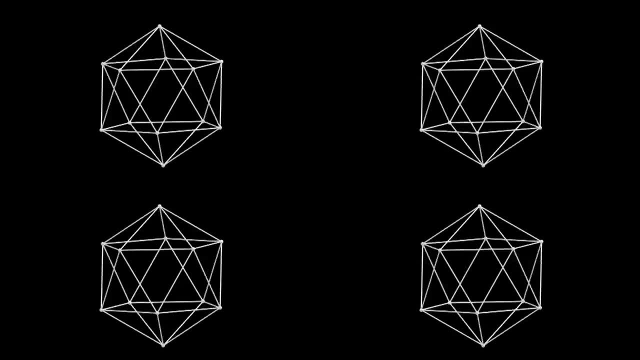 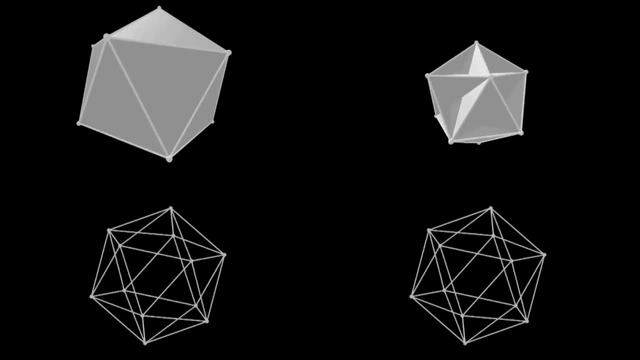 looking at their wireframes like this, they look exactly the same. two of them have flat faces which can be filled in, so we can see that this one is a nycosahedron and this one is a great dodecahedron. but for these two we can't do that. the best option I have is to just highlight one of. 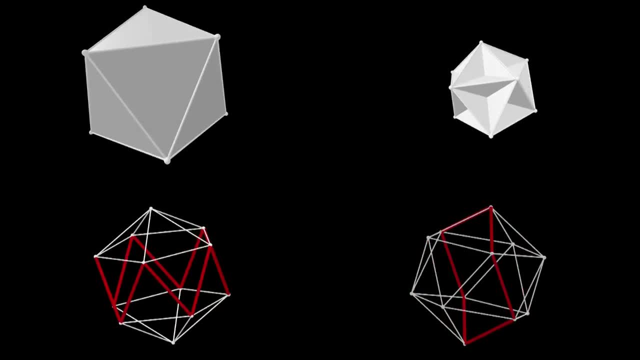 the skew faces so you can get a sense of the structure. and even then it's still super hard to not just see it as a nycosahedron. here let's have a quick montage of all of the petri polygons. 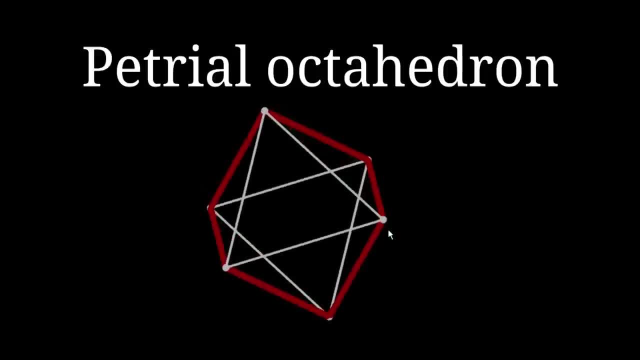 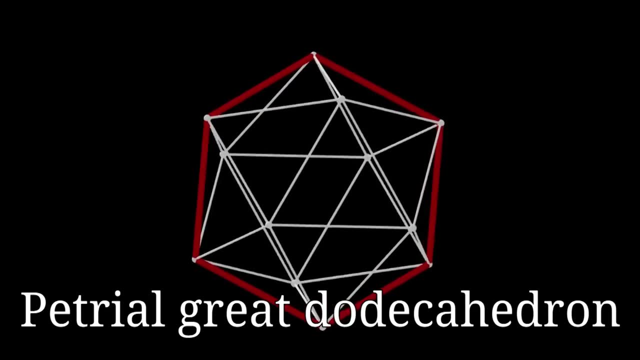 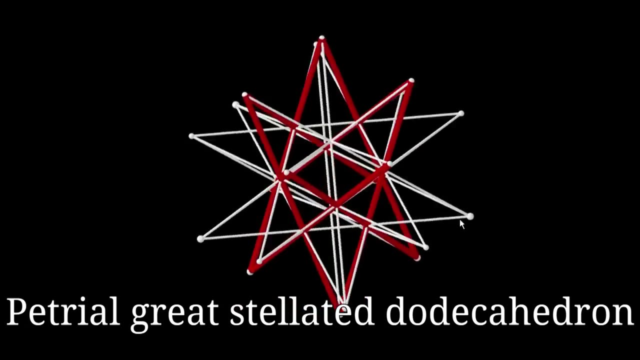 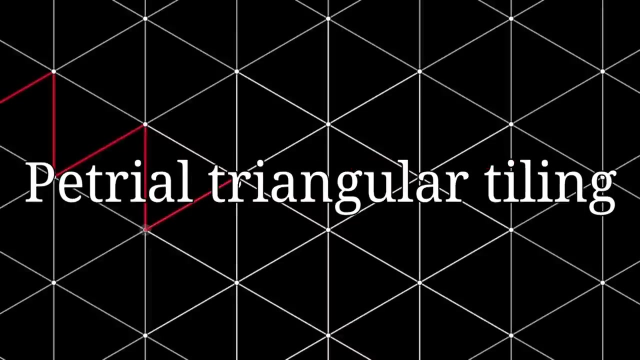 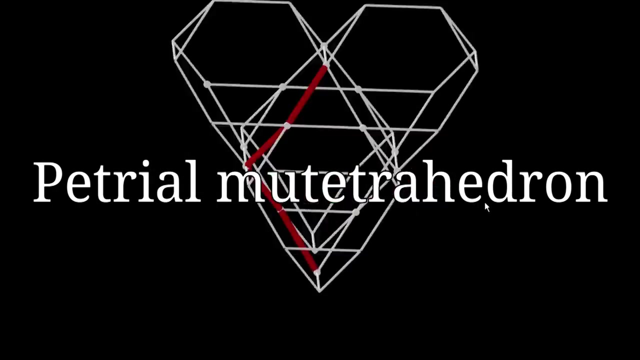 and how you can view them from a certain angle that makes them look more like normal, flat, regular polygons. anyway, with these petrioles we can now say that there are 30 regular polyhedra- at least there's 30 that have actual, established names. we have officially reached dark geometry. 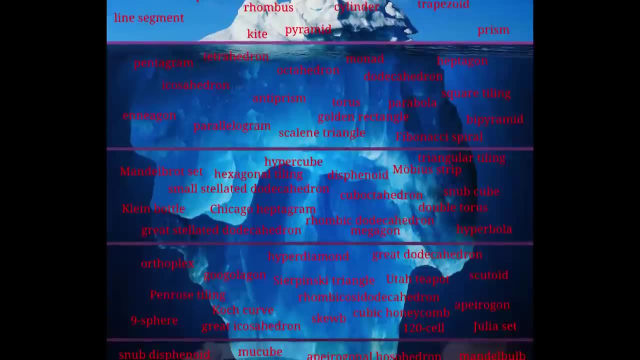 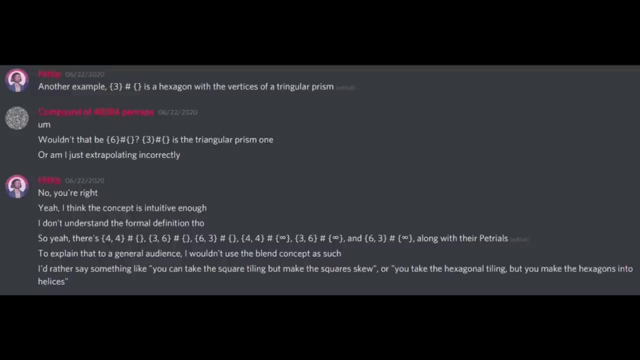 territory. researching the remaining 18 polyhedra was a complete nightmare. after sifting through pages upon pages of geometry jargon, I eventually was able to get some help from the fine people in the polytope discord server. I could not have done this without them. 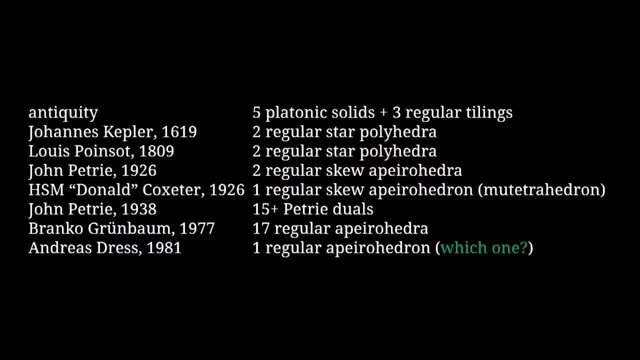 very frustratingly. I am aware that of these 18 polyhedra, 17 of them were discovered by Bronco Grunbaum in 1977, and one of them was discovered by Andreas Dress in 1981, and I have literally no idea which one Dress discovered most of my information about these. 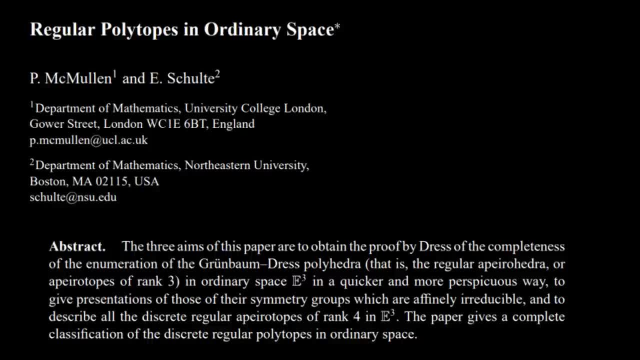 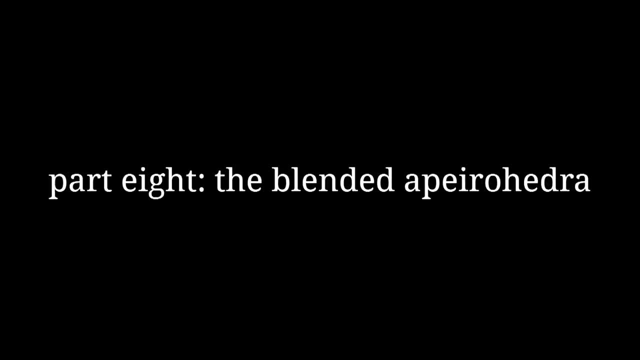 shapes comes from this paper from 1997, where McMullen and Schulte categorized the Grunbaum Dress polyhedra part 8.. the blended epirohedra 12 of the dark polyhedra can be created from the three. 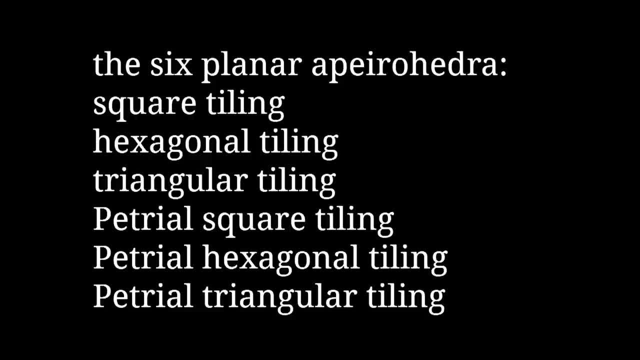 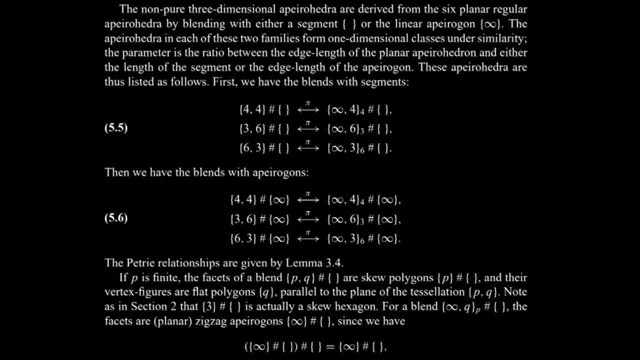 no, sorry, six flat epirohedra using a process called blending. each flat epirohedron can be blended with a segment or with an epirgon. this terminology is very confusing and it will be more helpful to think of these two kinds of blending as being completely separate. 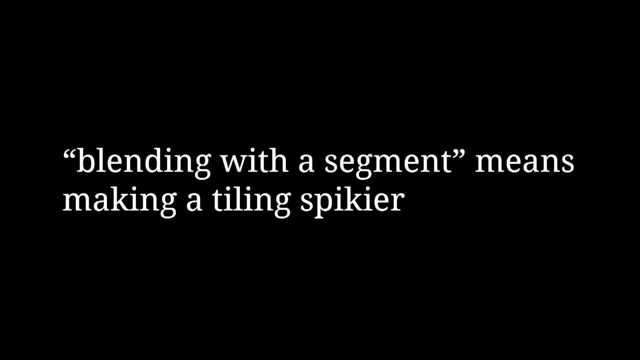 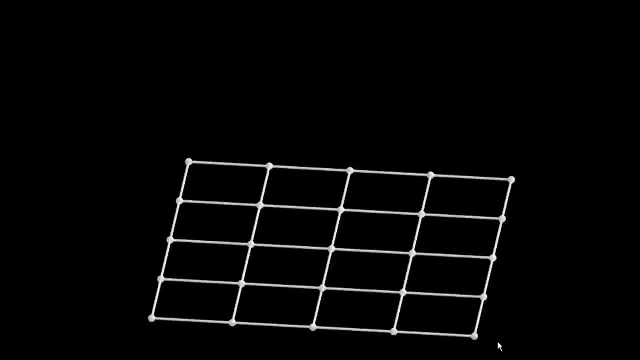 let's start by blending each of them with a segment, since that's easier. what that really means is that you're taking the flat epirohedron and making it spiky by lifting some of the vertices, just like how you can turn an epirgon into a zigzag in 2D and have it. 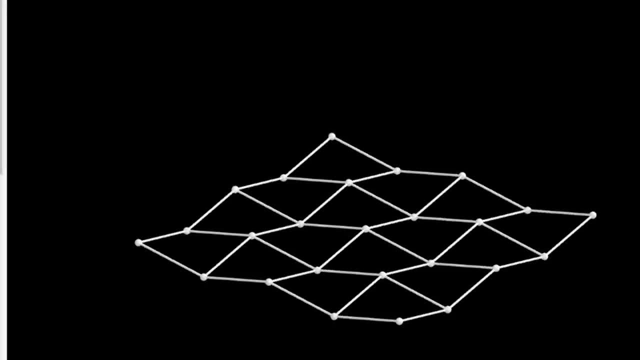 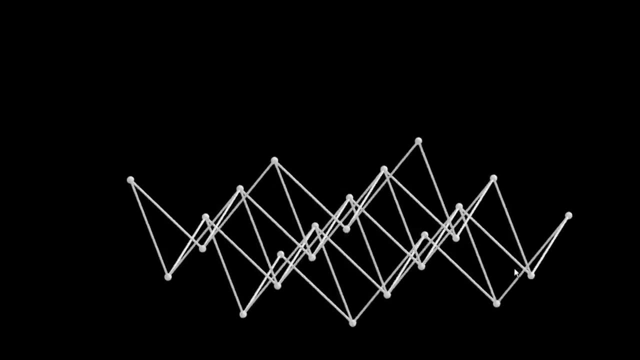 still be a regular polygon. making each of these tilings spikier doesn't stop them from being regular polyhedra. oh and for the petrioles, as you'd probably expect, you get stuff that looks the same but is technically different. standard deal for. 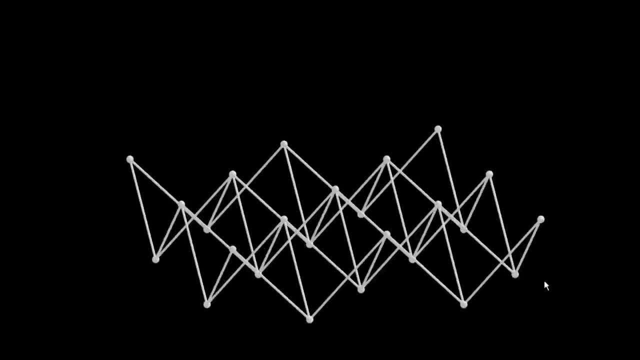 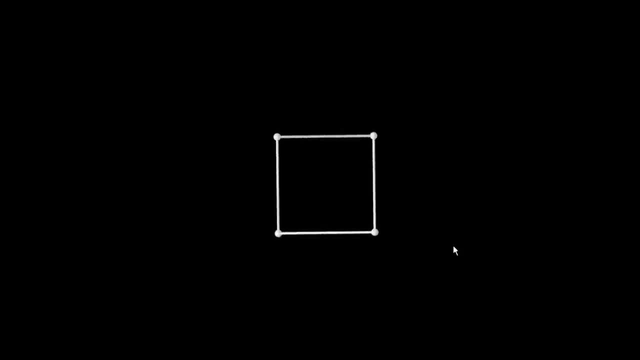 petrioles, really okay. now for the other type of blending: blending with an epirgon. to explain this, I'm going to have to first explain yet another type of regular polygon. take a look at this. you might think that this is a square, but look again. 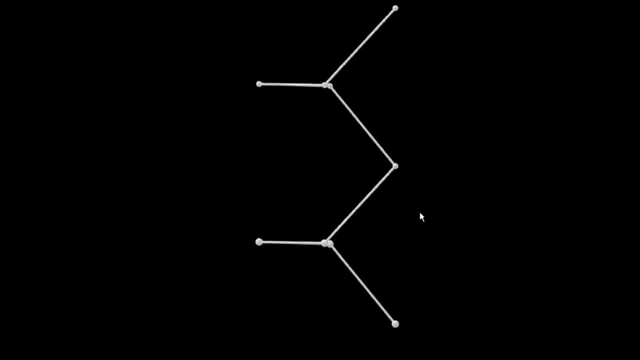 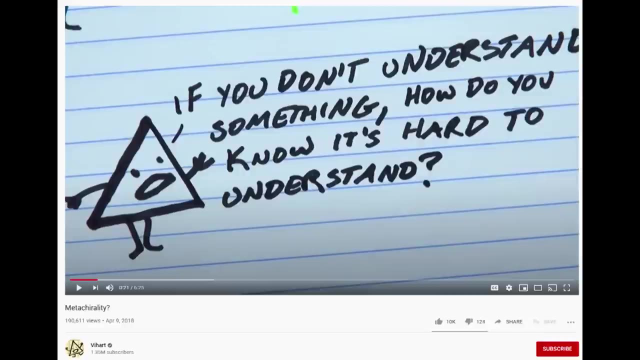 you're actually looking at an infinite spiral pattern of squares curling into the third dimension. this is a helix, and you can make a helix out of any polygon you want. this is a new polygon you want. Weihardt made a whole thing about this type of symmetry, which I highly. 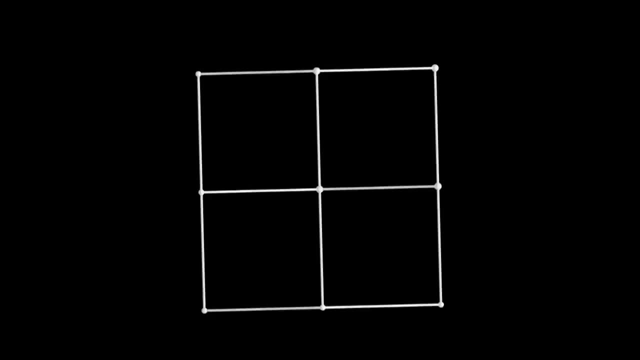 recommend so to create the other blended epirohedra, replace the faces of one of the flat tilings with helices, some being clockwise and others being counterclockwise, and once again there's petrioles that look the same, but aren't now none of these blended epirohedra actually. 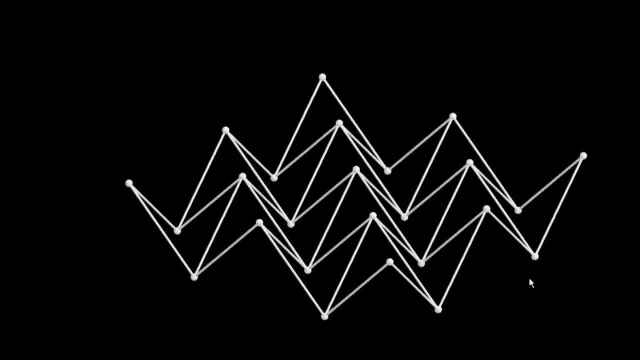 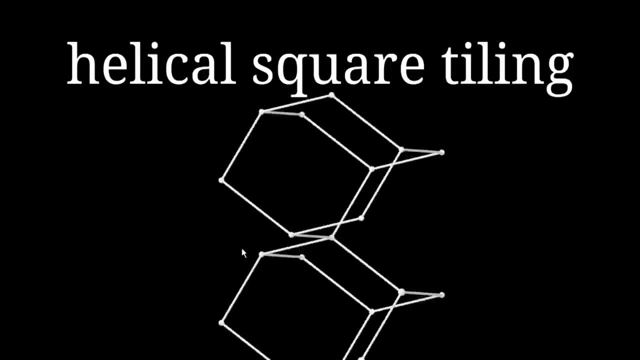 have names. I think it makes sense to call these ones, the endless spiky fields, the blended versions of the tilings, and to call these other ones the helical versions, since they're made out of helices. so these 12 infinite shapes get us up to 42 regular 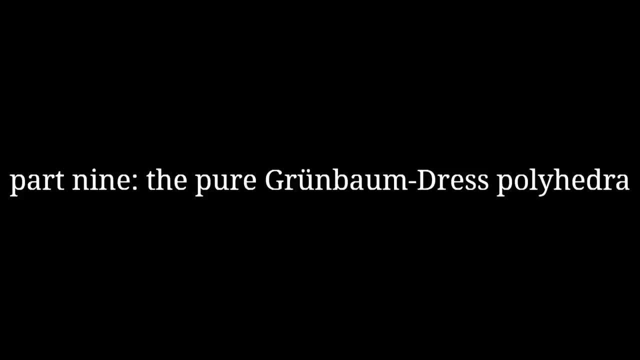 polyhedra. insert joke here. part 9, the pure Grunbaum dress polyhedra. we're almost done. there's only six regular polyhedra left before we're at the number promised in the video title. I'd like to introduce you to this chart. this is a chart featured in 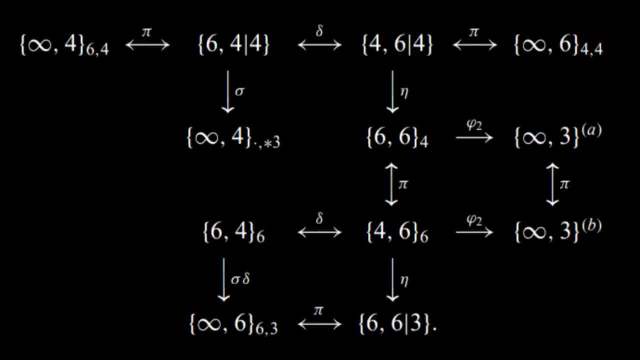 McMullin and Schultz's paper that I've spent a very long time trying to understand. it shows how all 12 so-called pure epirohedra are related to each other. take it all in. this is what I had to work with. half of these are the petri coccydor polyhedra and their petrioles. see, there's the mu. 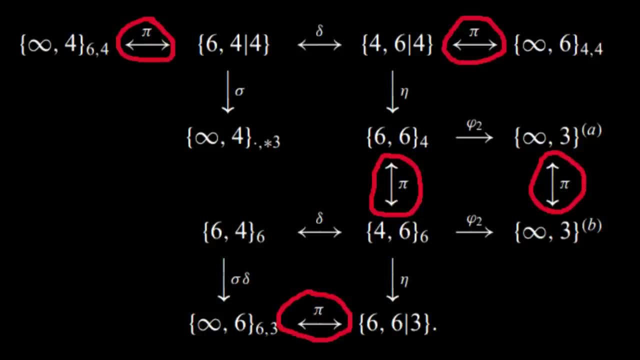 cube, mu octahedron and mu tetrahedral polyhedra. this is what I had to work with. half of these are mu cube, mu octahedron and mu- tetrahedral polyhedra. the letter pi here is used to. 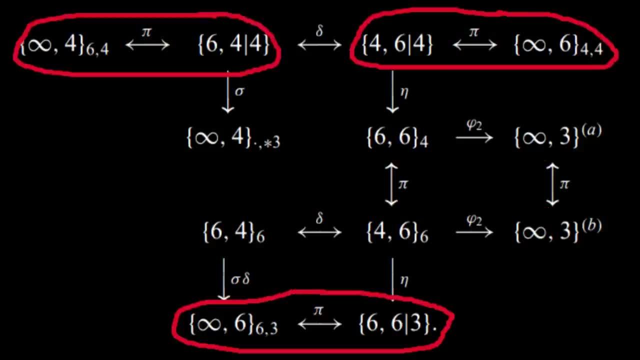 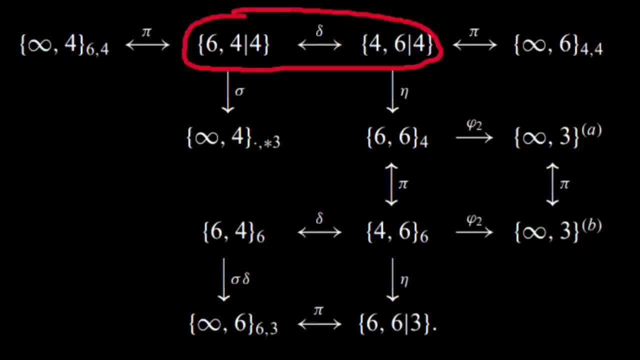 show which shapes are petrioles of each other. so these three are the petrioles of the petri coccydor polyhedra. there's also the letter delta, which connects the regular duals. so you can see that the mu cube and the octahedron are duals of each other. all we're left with is 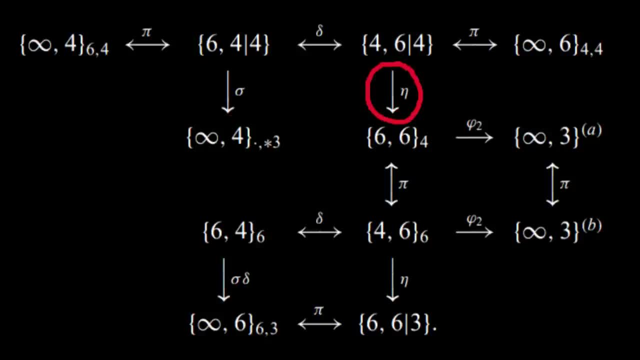 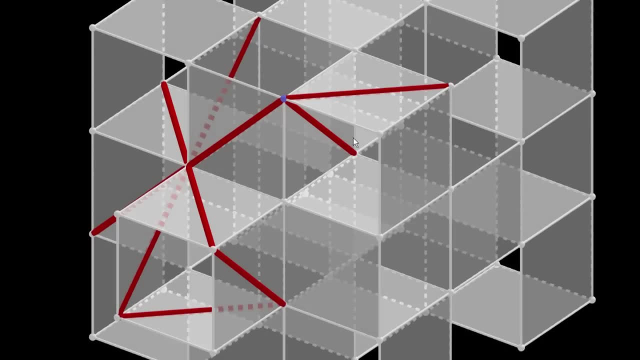 the six in the middle here. let's begin with this thing. the letter eta here means that it's derived from the mu cube by halving it. basically, you start with a mu cube and then you draw a line across the diagonal of each of the square faces in this symmetrical way, so that you have six of. 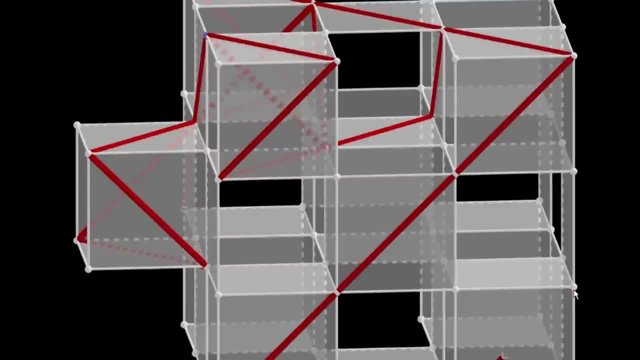 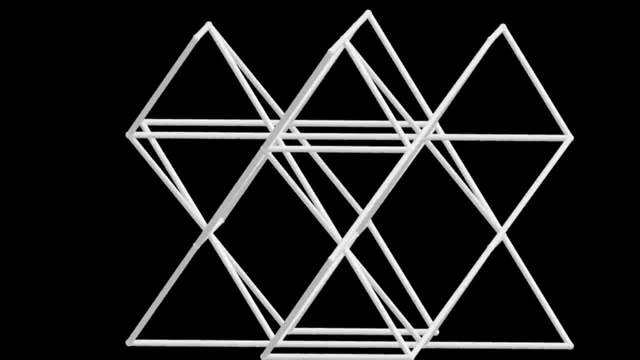 these new lines meeting at a vertex. now remove the original mu cube and just keep the new lines. what you're left with is, I guess, the result of having cut each of the mu cube's faces in half. I think it makes sense to call this a halved mu cube now if you follow along these edges. 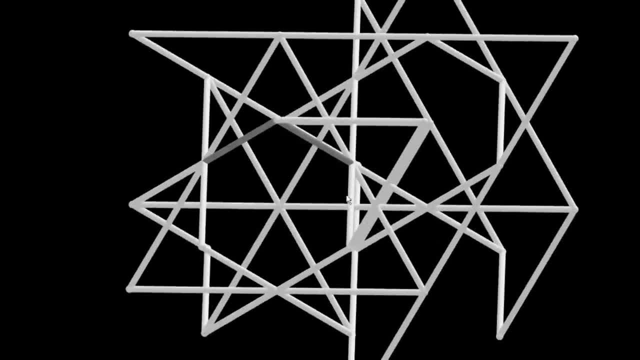 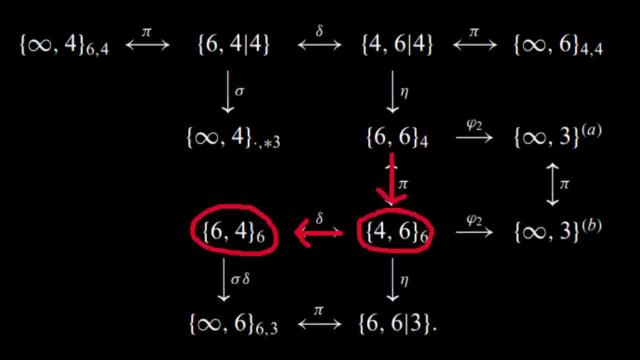 you'll see that this shape has hexagonal faces. that will be important anyway. you can also find the petri dual of this thing, which gets you back to halving square faces. from the petriol halved mu cube, you can derive this thing. remember the delta there means dual. 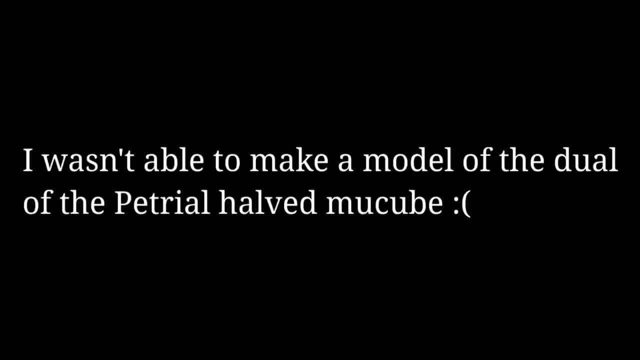 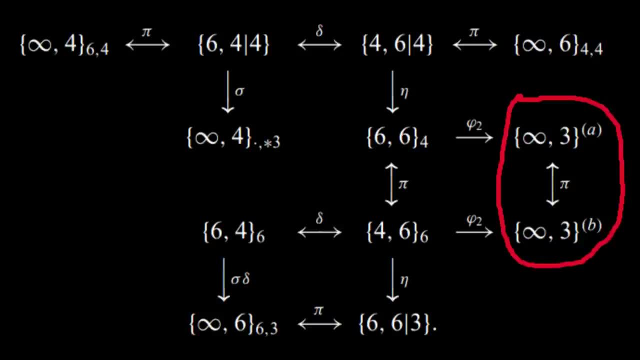 so we can find the dual of the petriol halved mu cube and we get this cool new shape with hexagonal faces. now let's go over these two on the right here. while they can be derived from the halved mu cube and its petriol, let's build them from the ground up instead. start. 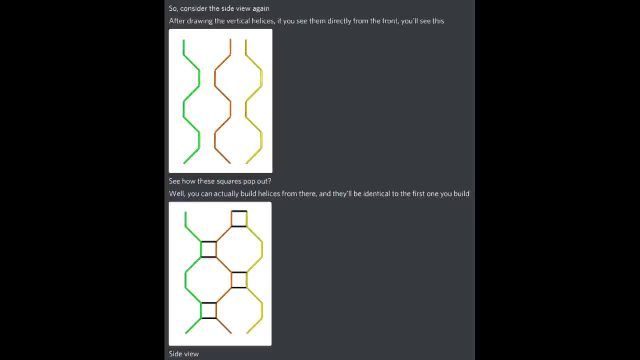 with some square helices. arrange the square helices in this pattern. now, if you view this thing from just the right angle, you'll see how these parts come close together. in fact, the distance between them is just right for you to connect them together and make some squares. 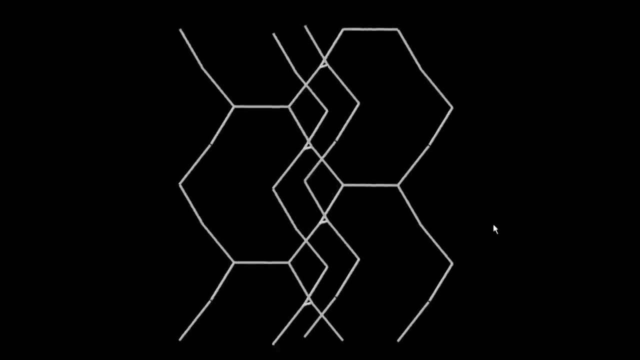 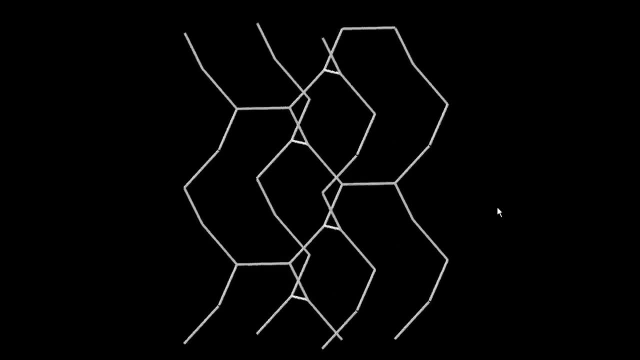 but actually they're not squares, because if you rotate it back around, what you've filled in is even more square helices. isn't that so cool? it's this infinite pattern of square spirals going in three directions at once. I'm going to call this thing the trihelical square tiling. the trihelical square tiling. 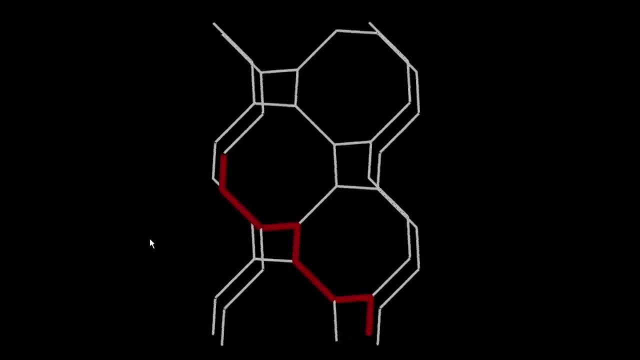 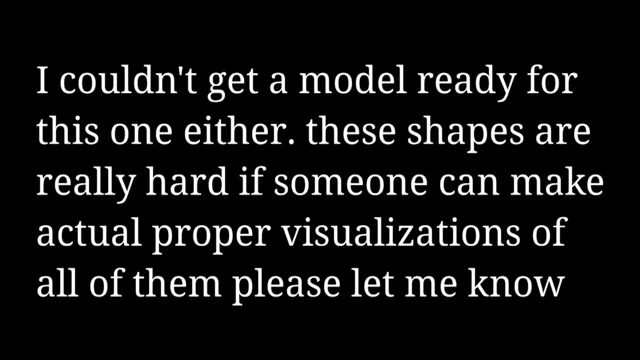 has a petriol which is made out of triangular helices that go in four directions at once, so it makes sense to call that one the tetrahelical triangular tiling. okay, last one begin with a mu-octahedron. each of the hexagonal faces can be turned. 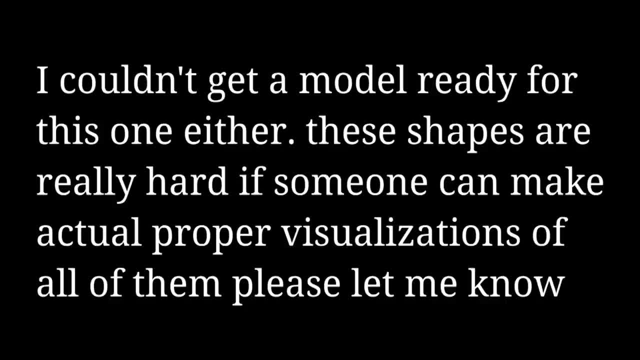 into a triangle by removing half of the vertices. now, looking at it from just the right angle, you can see that each triangle is part of an infinite tower of triangles. turn that infinite tower into a helix and you get the final regular polyhedron, the skew mu-octahedron. 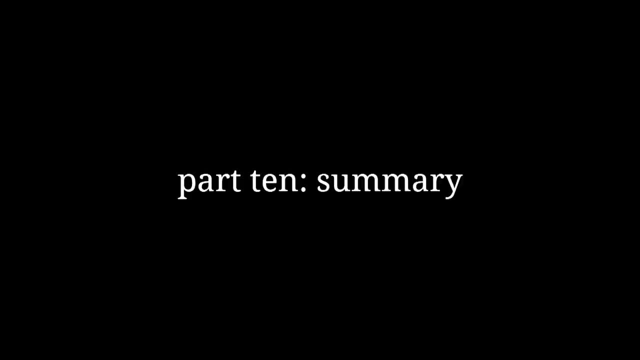 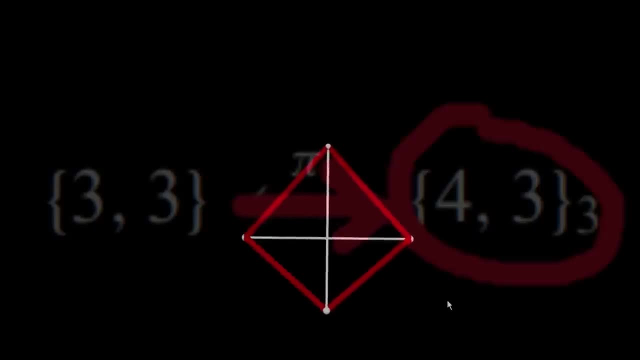 part ten summary. there are 48 regular polyhedra, 18 of which are finite. the simplest one is the tetrahedron. by looking at it from a different perspective, you can construct the tetrahedron's petri polygon. 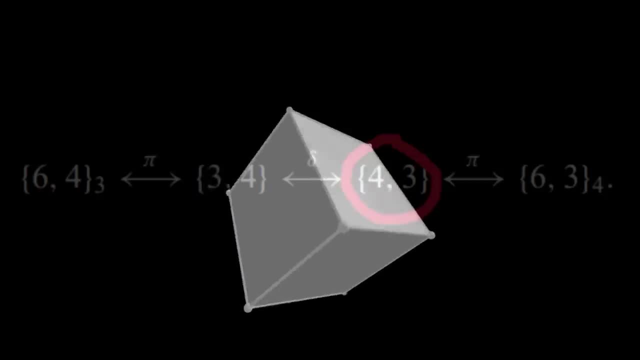 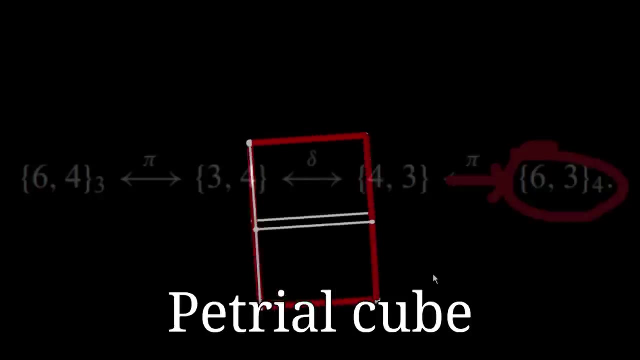 a skew square and with that the petriol tetrahedron. another simple, regular polyhedron is made out of squares and it's called a cube. the cube has a dual called the octahedron, and both polyhedra have petriols: the petriol cube and petriol octahedron. 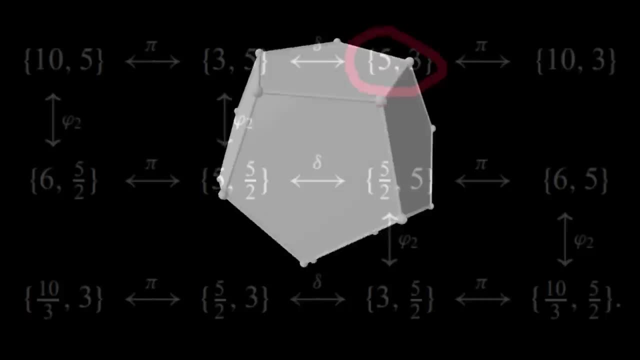 both of which have skew hexagonal faces. another regular polyhedron is the dodecahedron, made out of pentagons, its dual and greatening. the icosahedron and great dodecahedron have the 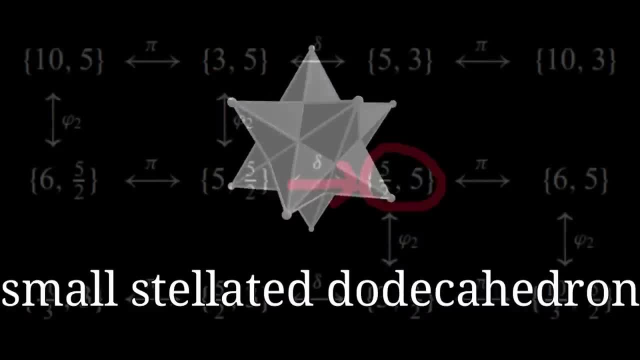 edge arrangement. and the same is true of the great dodecahedron's dual, the small stellated dodecahedron, and the icosahedron's greatening, the great icosahedron, the great icosahedron also. 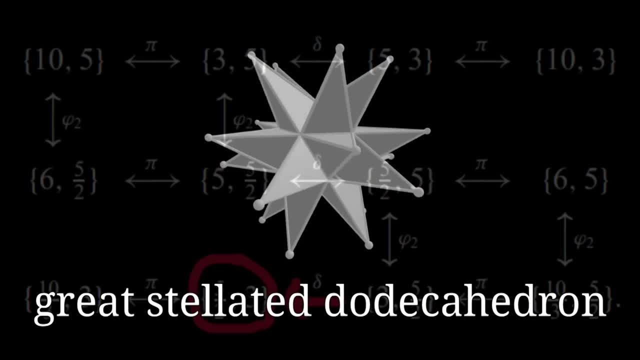 has a dual, which is another stellation of the dodecahedron, the great stellated dodecahedron, the petriol dodecahedron, petriol icosahedron, petriol great icosahedron and petriol great. 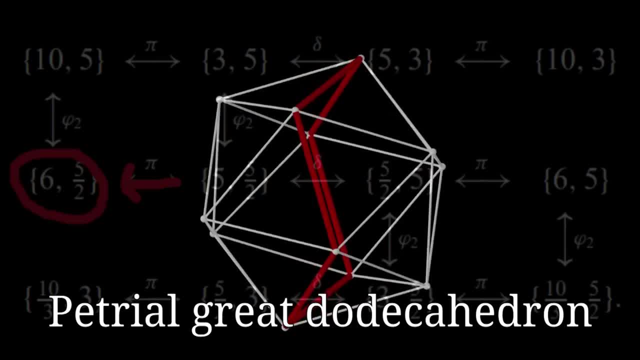 stellated dodecahedron. all have skew decagons as faces and the petriol great dodecahedron and petriol small stellated dodecahedron have skew hexagonal faces. the other 30 regular polyhedra. 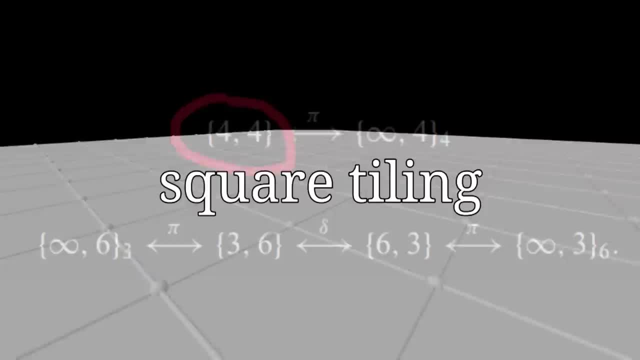 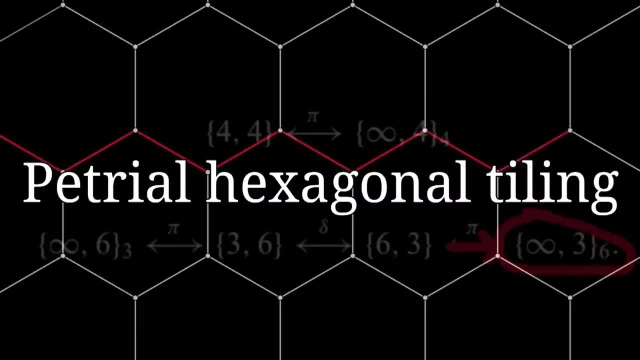 are all infinitely large. six of the regular epirohedra are flat tilings: the square tiling, its petri jewel. the petriol square tiling. the hexagonal tiling and its jewel. the triangular tiling and their petri jewels: the petriol hexagonal tiling and petriol triangular tiling. 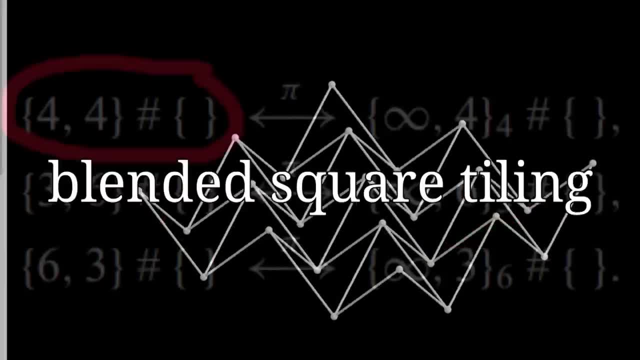 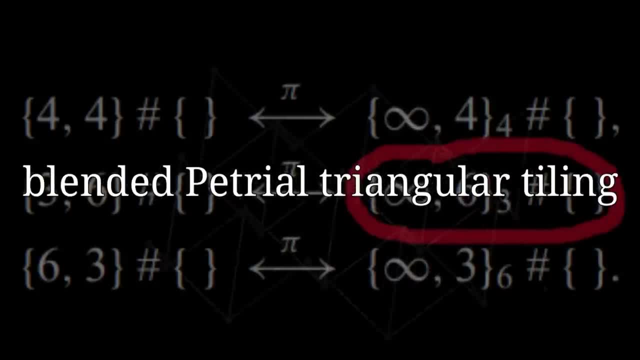 all six regular tilings can be blended, either with segments forming the blended square tiling, blended hexagonal tiling, blended triangular tiling, blended petriol square tiling, blended petriol hexagonal tiling and the blended petriol triangular tiling, or with a pyragons. 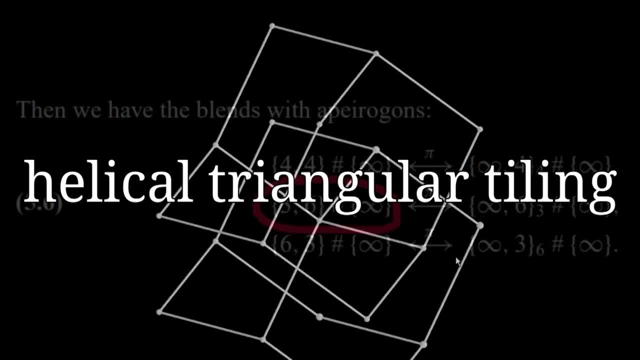 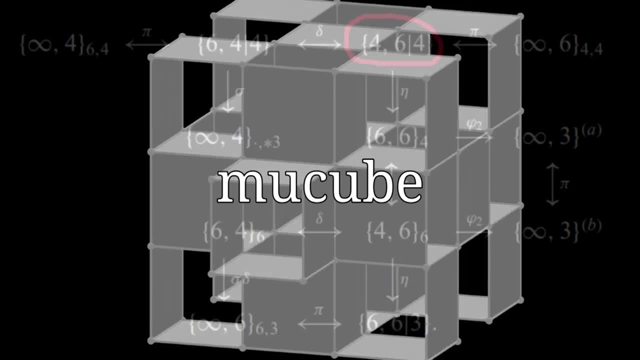 forming the helical square tiling, helical hexagonal tiling, helical triangular tiling, helical petriol square tiling, helical petriol hexagonal tiling and the helical petriol triangular tiling. a mu-cube can be constructed by removing some of the faces of a cubic honeycomb. 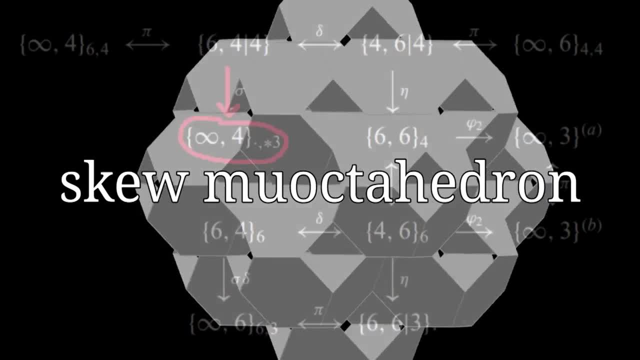 its dual, the mu-octahedron, can be skewed to form the skew mu-octahedron. the mu-cube and mu-octahedron both have regular petri-duals: the petrial mu-cube and the petrial mu-octahedron. 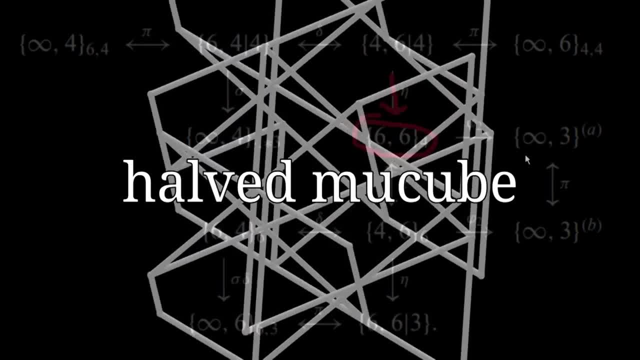 if you cut the mu-cube's faces in half, you end up with the halved mu-cube. the halved mu-cube and the petrial halved mu-cube can be faceted into the tetrahelical triangular tiling and the 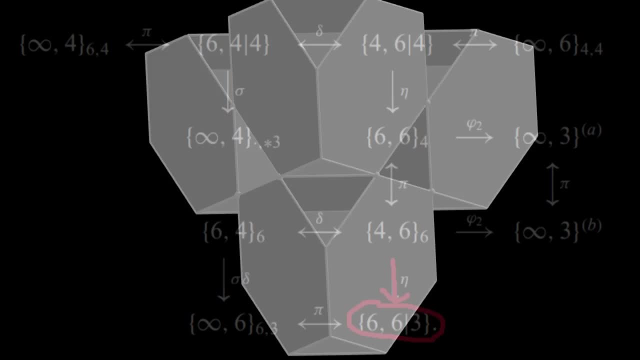 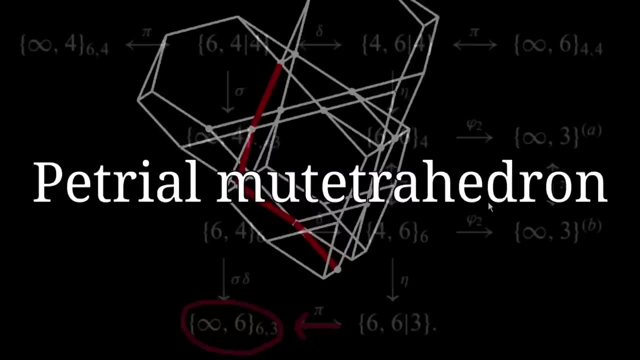 trihelical square tiling respectively. the petrial halved mu-cube can itself be halved to form the mutetrahedron, and the petrial mutetrahedron can be derived either as the petri-dual of the mutetrahedron or as a skew-dual of the dual of the petrial halved mu-cube. 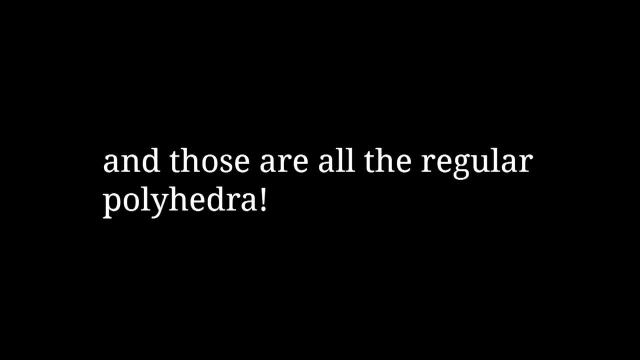 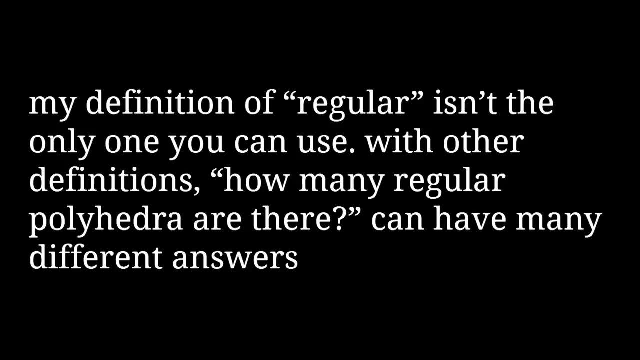 and those are all 48 regular polyhedra, or are they? I still made a lot of assumptions in the definition of regular I used for this list. I assumed that a regular polyhedron can't have two faces, two edges or two vertices in the same place. I assumed that the faces of a regular 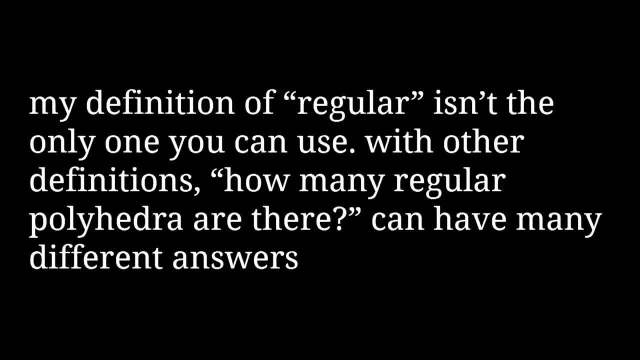 polyhedron must all be connected. I mean heck. I assumed that a regular polyhedron has just two faces and two edges and two vertices in the same place. there are no polyhedron has to fit in 3D Euclidean space. removing any of these assumptions makes the 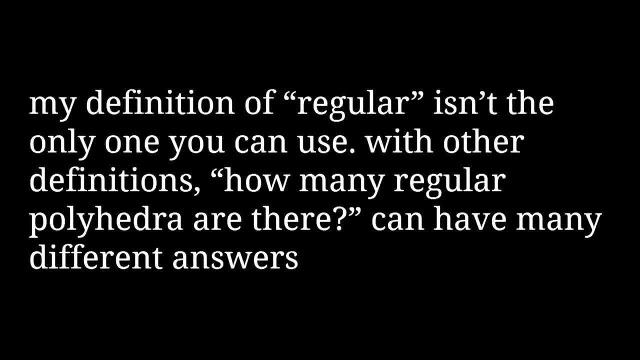 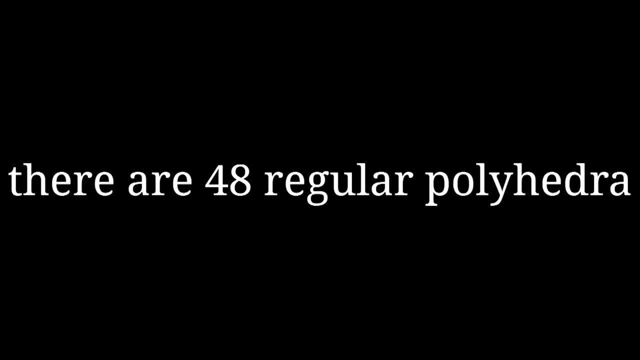 question much harder to answer definitively and the version of the question I answered here was already hard enough. still, I think these were all reasonable restrictions to include and if you agree with me, then there are 48 regular polyhedra. I've been jan.